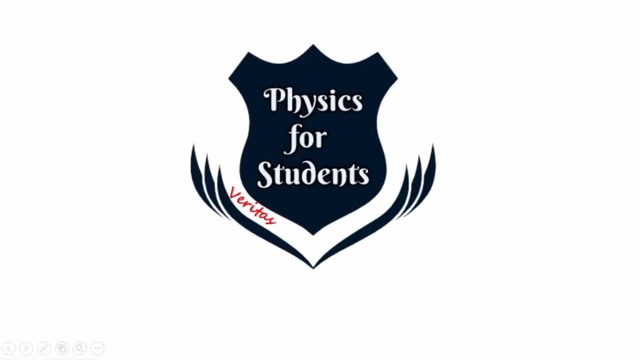 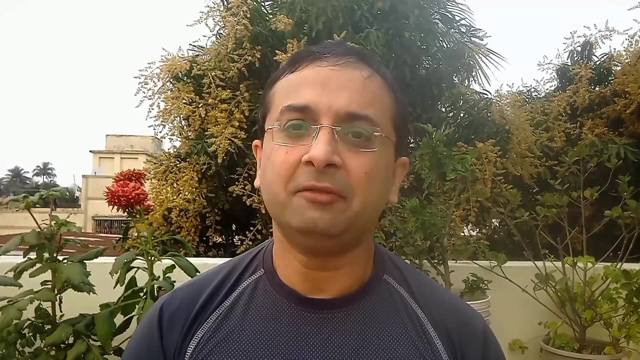 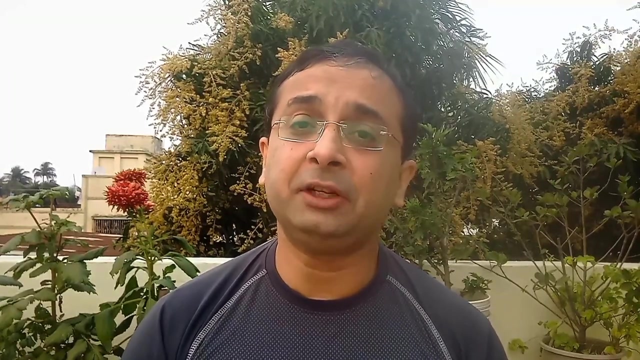 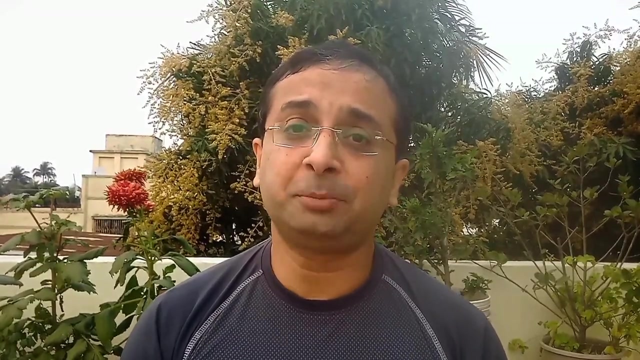 Mathematical symbols. Ever since the dawn of human civilization, we have seen the usage of different mathematical symbols, signs and anagrams, which are found engraved in pillars, caves, tablets and on different stones. If we go back to the ancient Greek, Mesopotamian and Sumerian civilization, we find the usage of different types of symbols. 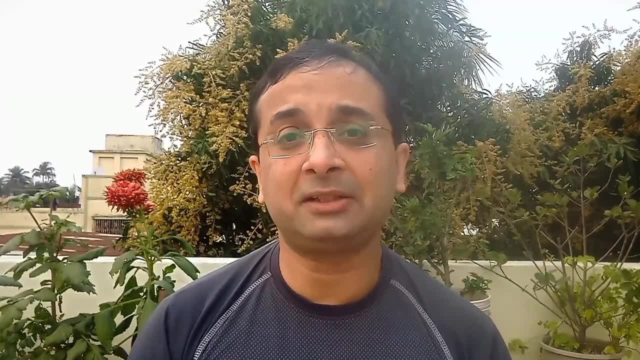 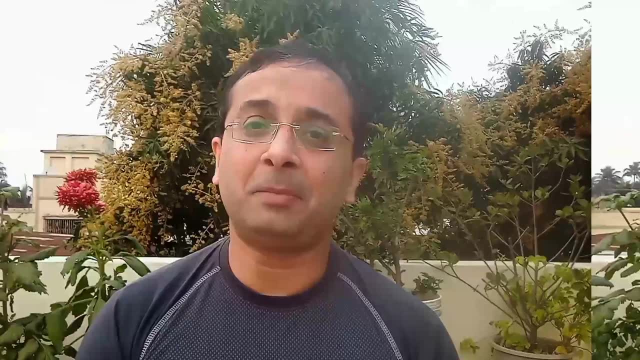 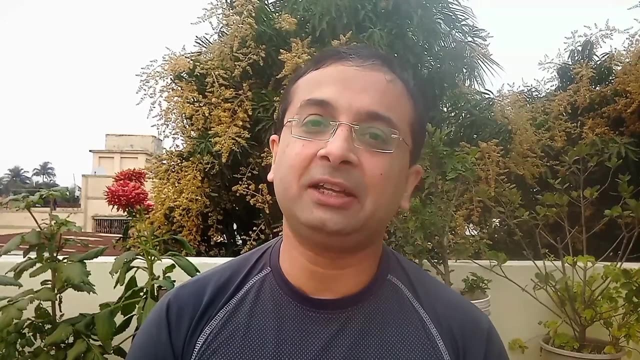 As with the advancement of human civilization, these mathematical symbols are later being used in science, astronomy, astrophysics and different branches. Welcome to my channel, Physics for Students. My name is Sean Up and I welcome you to a fresh new series of lectures on discovering mathematical symbols. 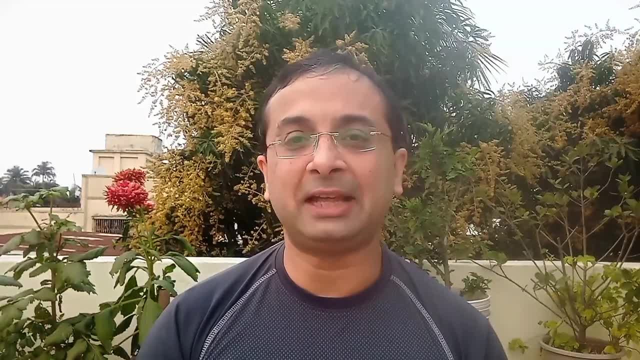 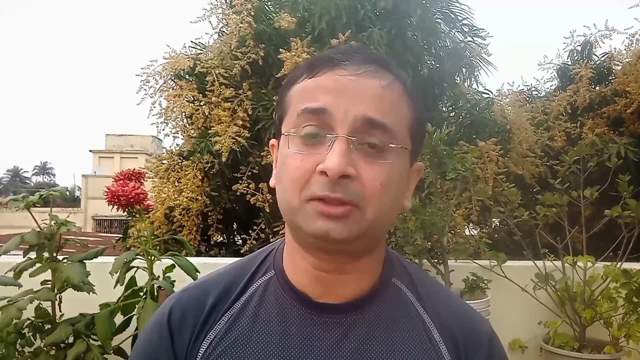 In this due process of this lecture, I would like to introduce you to a few of my students. In this lecture, what I am going to do is that we are going to dig and we are going to find what was the origin of these mathematical symbols. who discovered those symbols? or we can also find out the civilization which was responsible in discovering those symbols. 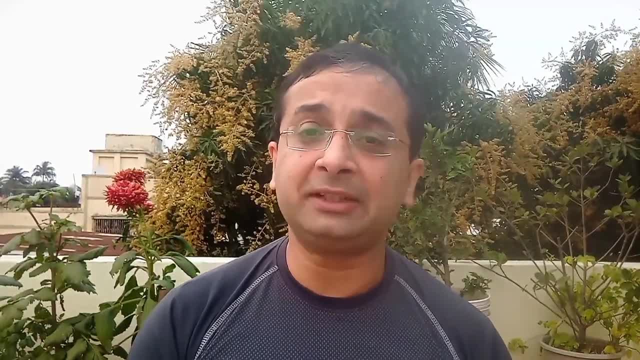 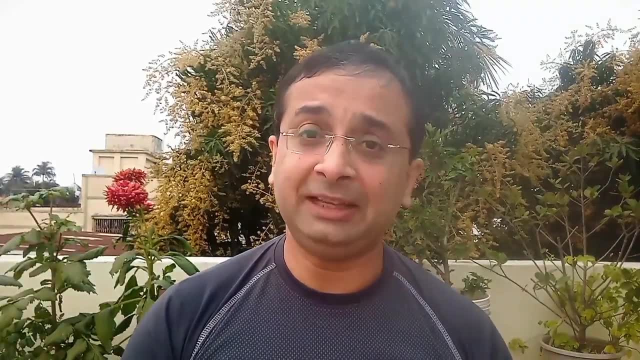 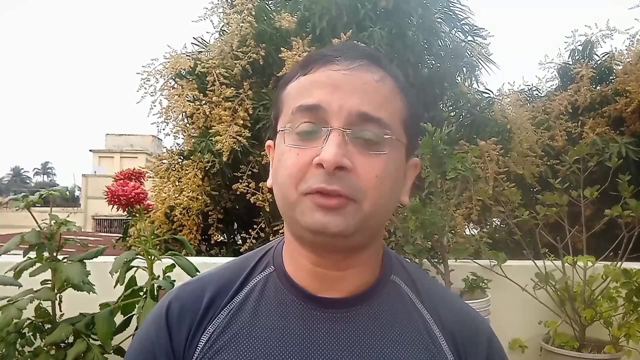 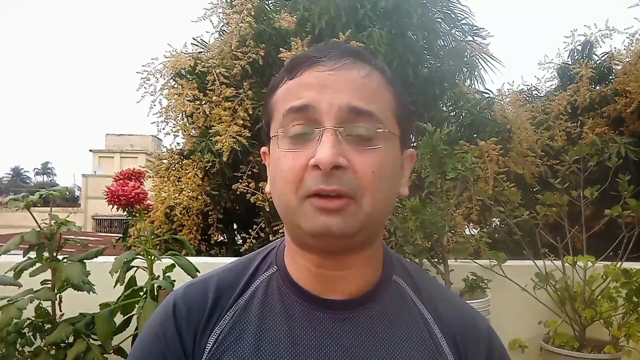 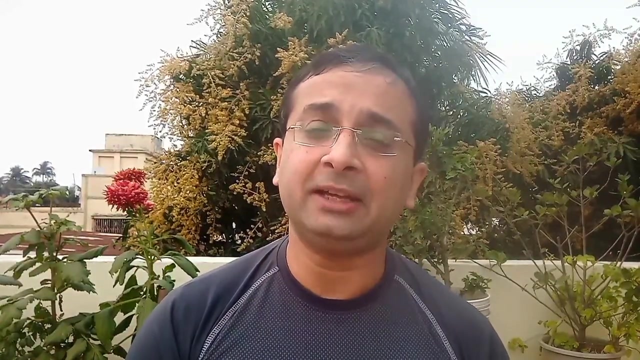 In due course of time, we will also find out how these symbols are being used. Is it that plus and minus and subtraction and division is only being used in the general sense, or they have higher and better uses in advanced mathematics? My request to all of you is that in due process of time, we will also find out that we are not, you know, using the general field of mathematics, but we have to go and learn certain advanced fields of mathematics, which includes number theory, Galois theorem, group theory, category theory and further on. 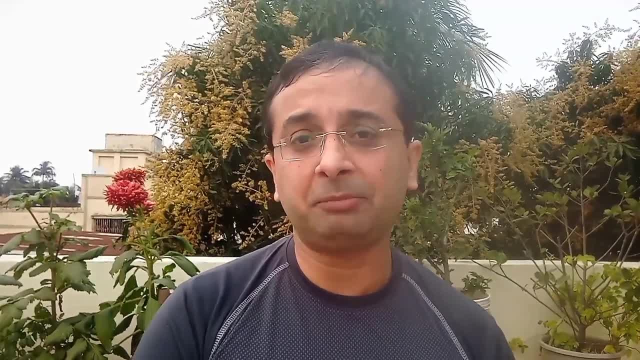 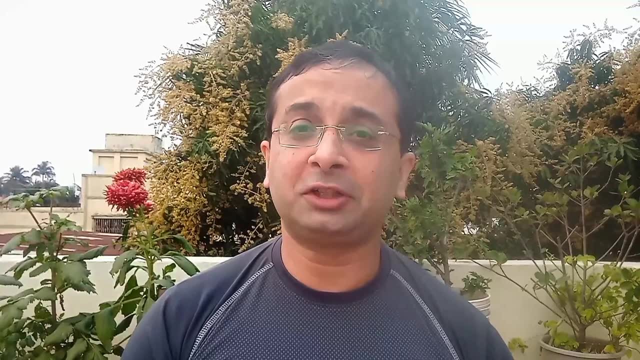 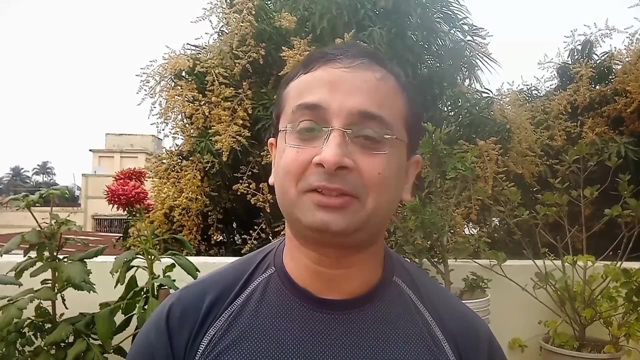 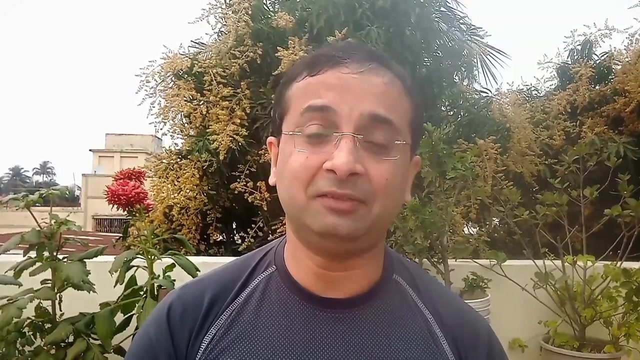 Because I would really like to show you that, apart from the general notion of those symbols, what are the other areas in mathematics and how they are being used. So just stay tuned And just be ready to plunge into the adventure of discovering mathematical symbols, going back to the past, discovering the past and knowing the real reason, the person and the civilization responsible for developing these mathematical symbols. 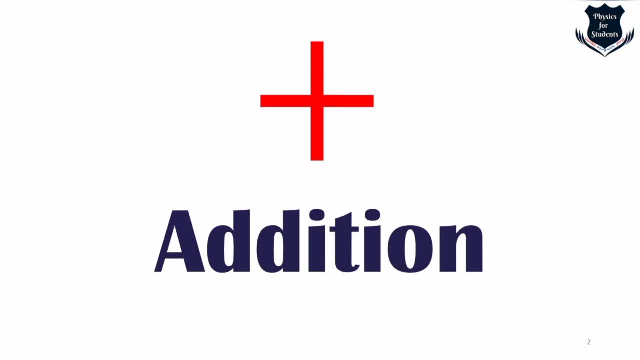 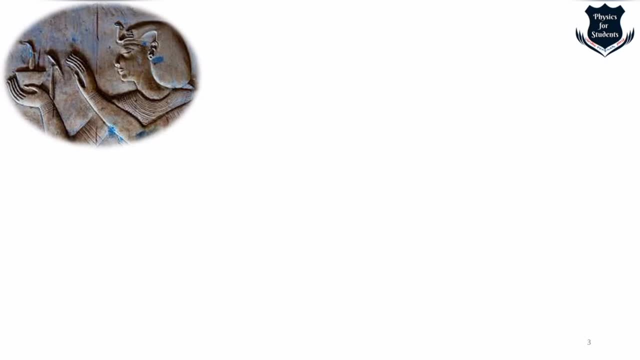 So first we look forward, the basic symbol of arithmetic operation, which is the addition. Now the symbols. as we know, we go back to the ancient Greeks. But the Greeks, They used these symbols not for addition, subtraction, division and multiplication, but they were used for esoteric cult symbols about combining of the feminine with the masculine. 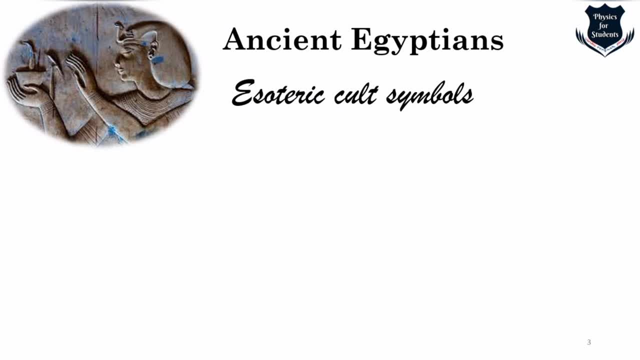 You can state it in another way, that it is combining a masculine god with a feminine goddess. So this Hansen belief was tied up with the religious philosophy that a mortal human woman could become a goddess And a mortal human man could become a god through a process of magical transformation. 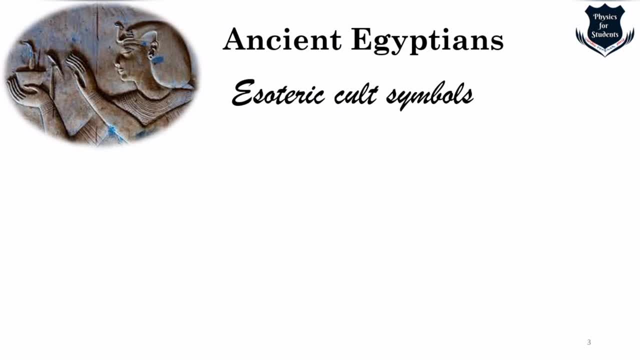 So the ancient Egyptians using the esoteric cult symbols and they used to worship the mathematics which you have seen earlier in my videos where I have spoken about the Pythagorean argument that numbers were independent of reality and numbers were worshipped as god and goddesses. 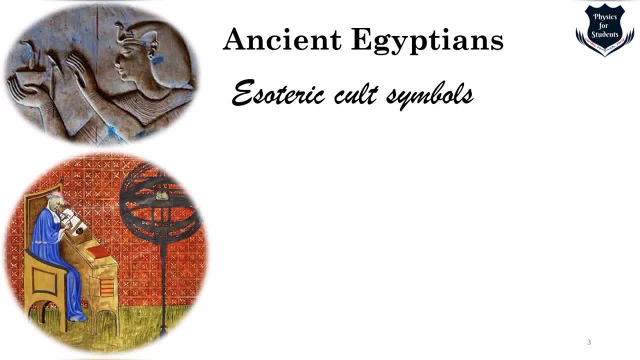 Now, history dates back to the early 20th century. History dates back to one of the influential French philosopher of the later Middle Ages, Nicole Orison, or Nicolas Orison Well, not much is known about his family. He studied arts in Paris and was born in Normandy. 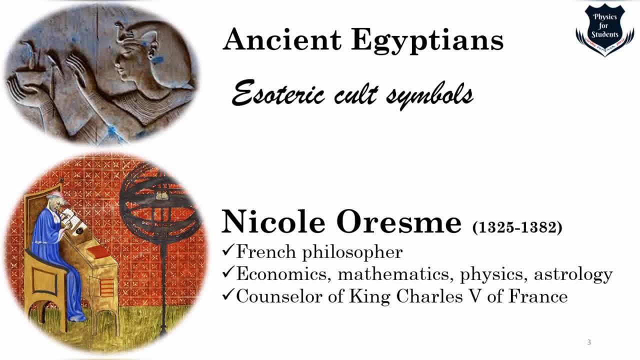 In 1348, he was a student of theology in Paris And in 1356, he received his doctorate. So here, right on your screen, I have just given you basic few points. So Nicole Orison, economics, mathematics, physics and astrology teacher, and he was a counselor of King Charles V of France. 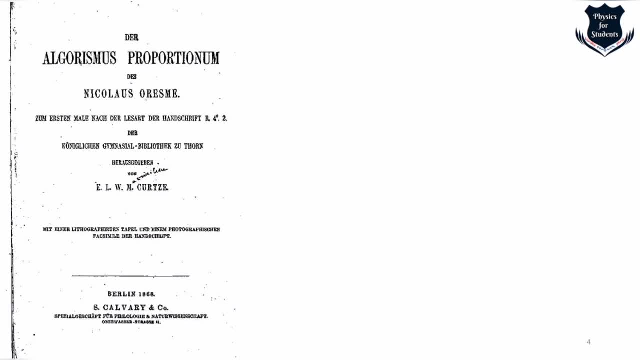 Later part we find one important book of Orison, Allegorismus Proportionum, believing to have written between 1356 and 1361. And here we first find the usage of plus. The symbol appears in manuscript of this work which is believed to have been, you know, written in the fourth century. 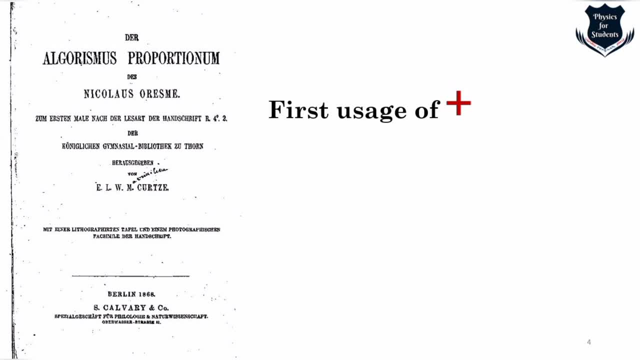 14th century, but perhaps by a copyist and not by Orison himself. Now, this usage of the plus sign was used by the Latin word et or, at, which means and. And. as you see that Orison used the word at, that signifies some or addition, in the following lines: 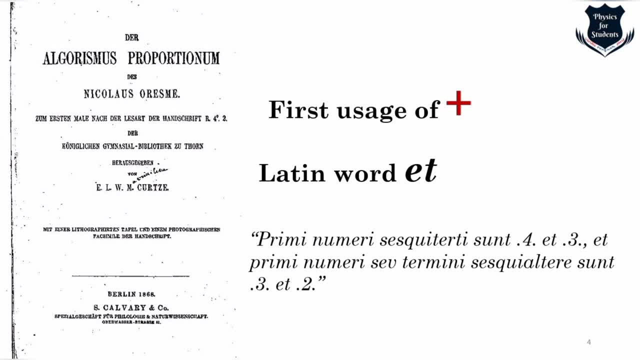 To be very honest with my poor Latin, I won't go forward in reading this line, But those who are aware about Latin, you can go forward And read this line. As you can see, he used this word for et three, et primi numeri and so on. 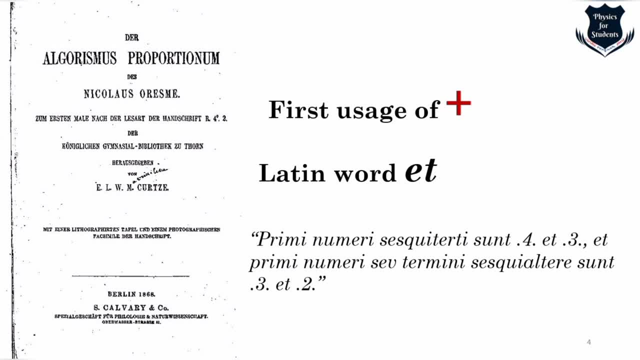 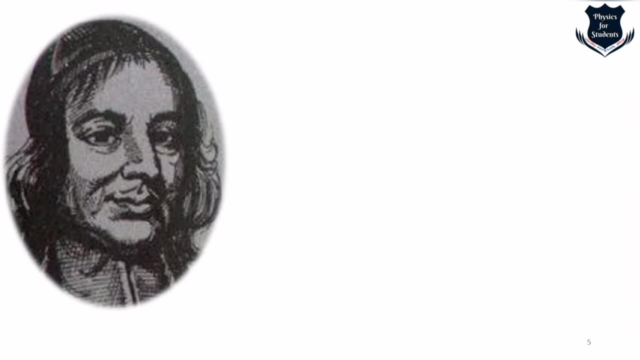 So this book very important in our learning of history, that the first usage of plus which is used as et, which means addition, Johannes Wildman, or Johannes Widman, was a German mathematician who is best remembered for an early arithmetic book. 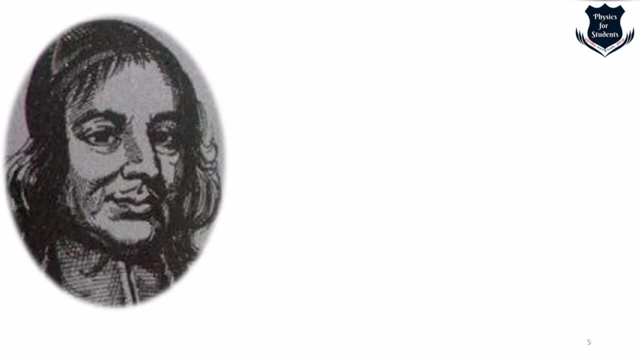 which contains the first appearance of plus and minus signs. Johannes Widman, whose name is also written as Weidman, attended the University of Leipzig, and his name appears on the list of those registered for the winter semester of 1480 as Johannes Widman de Aigre. 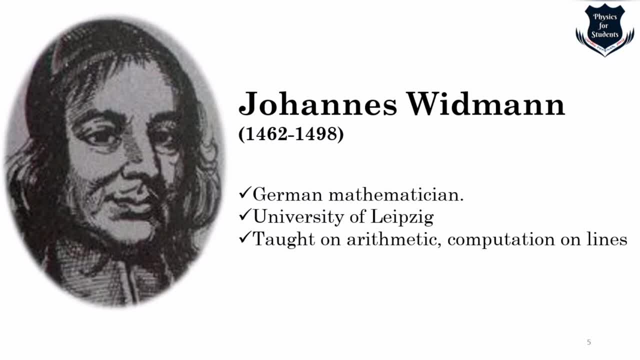 He graduated with a first degree in 1482 and he continued to study for a master's degree, being allowed to live outside the dormitory. His master's degree was awarded in 1485, and then he taught at the University of Leipzig on the fundamentals of arithmetic, computation of lines and algebra. 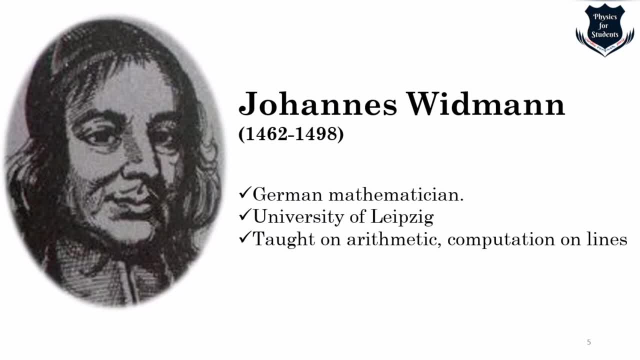 His lectures were advertised and students were invited to attend. So you see I've just given a few points. He was a German mathematician teaching at the University of Leipzig, and what are the essential areas that he taught? Now, Widman's 1486 algebra lecture was the first to be given in Germany on that topic. 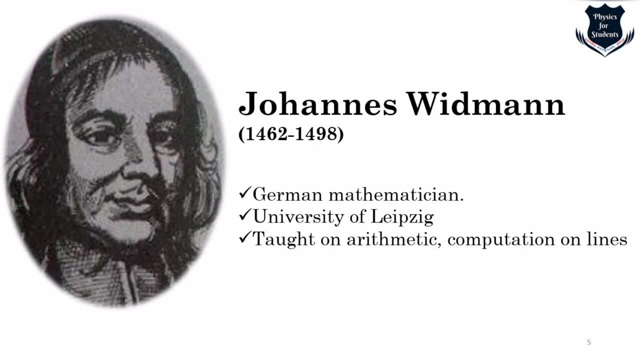 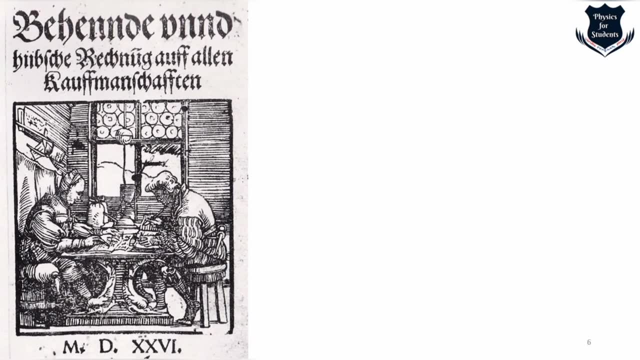 and amazingly it still survives a notebook of the student who attended. The name of the book, I won't dare to pronounce it. it is in German. This is basically the book. it is an early arithmetic book: Behend und Hupsche. whatever be, I would be very wrong if I pronounce it with a wrong grammar or a wrong German pronunciation. 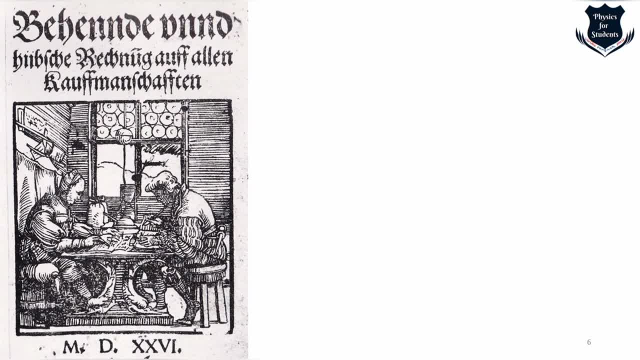 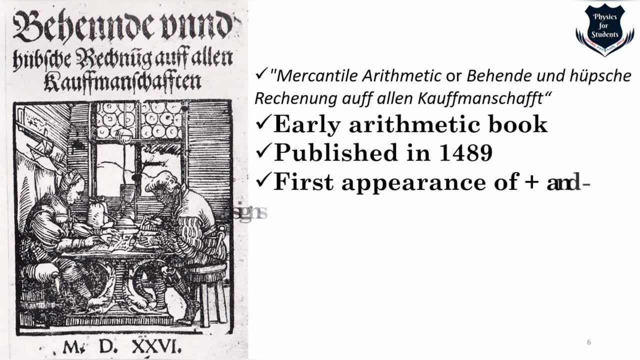 which is more or less. if it is translated in English. it means nimble and pretty account on all merchants. It was published in German in 1489, and that Widman was best remembered. This book has become famous since it contained the first appearance of the plus and minus signs for addition and subtraction. 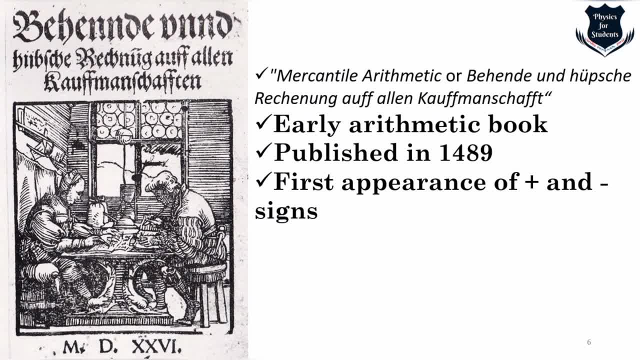 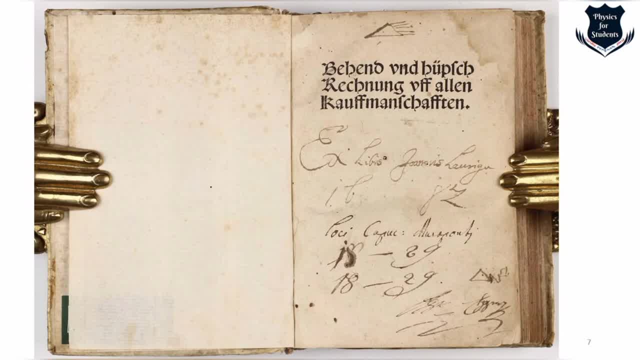 Now, as you can see, this is the cover of the early book and Widman actually, actually. yeah, so you see this. this is the picture of the book which you have taken, the first page of Widman and the name of the title of the book. 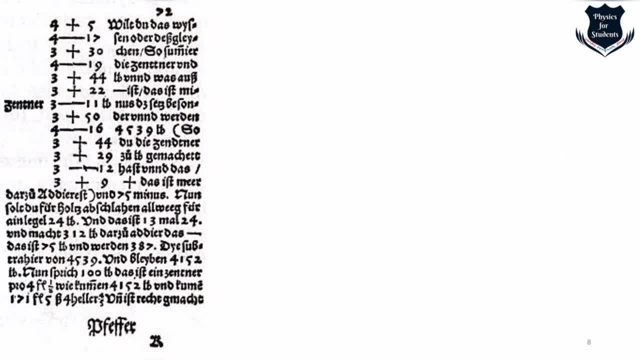 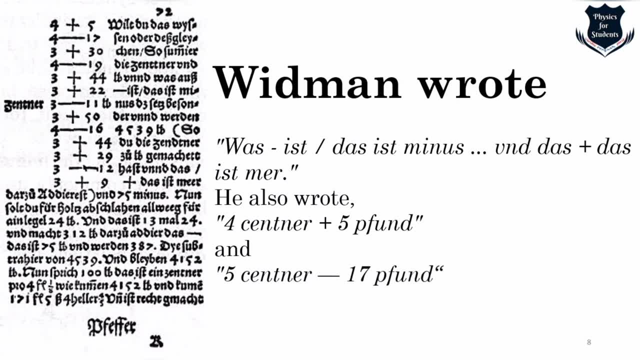 Most importantly, this is actually one of the excerpt of the book, and in here Widman wrote this in German right. So four centenar plus five. whatever it is, you can more or less understand. it shows the excess or deficiency in the weight of boxes or bales. 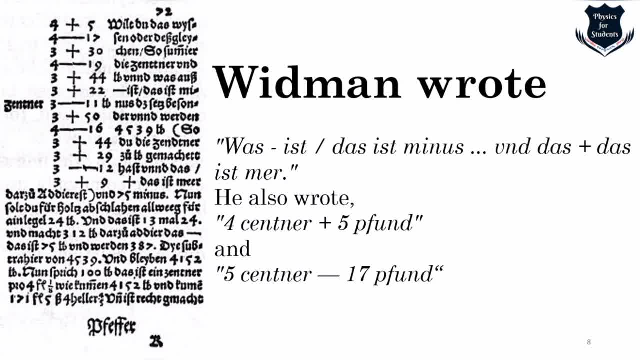 So as because it was merchant and it was related to trading, so it signified the excess or deficiency in the weight of boxes. Now, here I would like to draw your attention to another famous historian: Florian Cagiori, the famous Swiss American historian, mathematician. 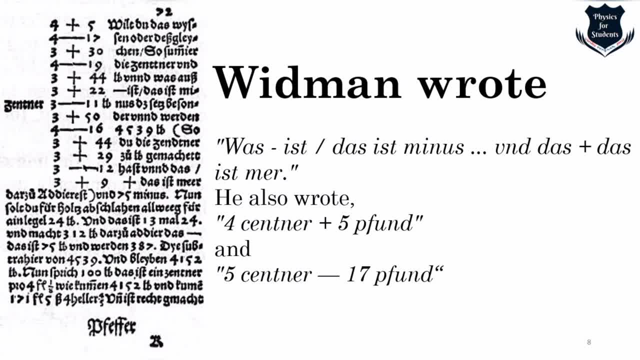 and he said there is a clear evidence that, as a lecturer at the University of Leipzig, Widman had studied manuscripts in the Dresden Library in which plus and minus signs signify operations, some of these having been written as early as 1486, right. 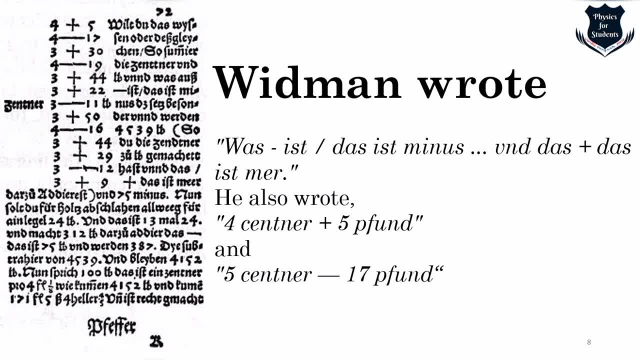 So Cagiori, who is known, you all know, for his famous book on discovering the history of mathematical symbols. he says that he studied in the Dresden Library, in which the plus and minus signify operations, and it is written as early as 1486. 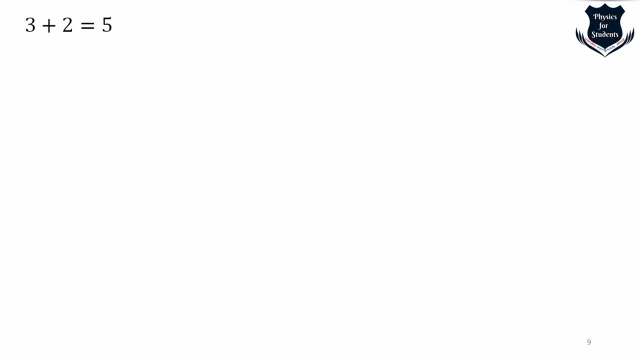 So let us look now into the usage of the symbols other than 3 plus 2,, 5, which we all know It is actually used. what is meant by disjoint union? So you get a U sign with a plus at the middle. 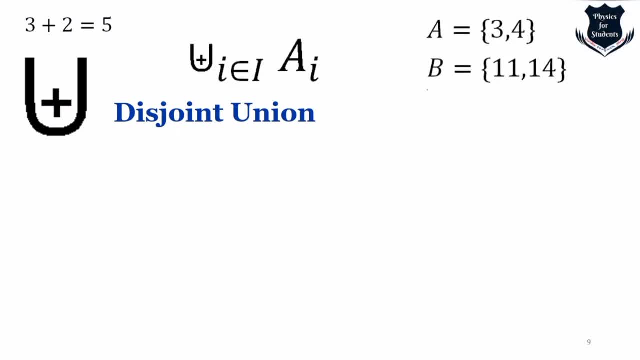 and this is the usual sign of disjoint union. Now, if I go forward and explain to you what is a disjoint union, we get a set A equals to 3 and 4, B equals to 11 and 14, and we try to join it right. we add up all the elements of the set A, B equals to 11 and 14,. 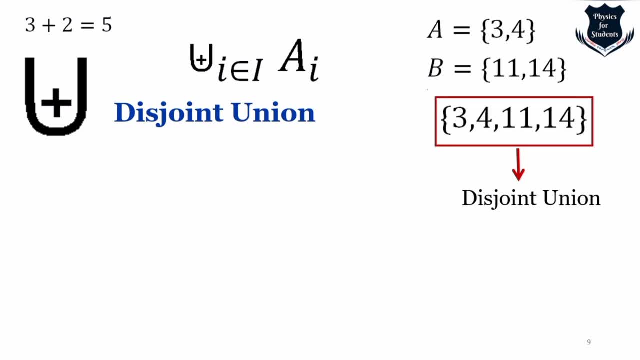 and we try to join it right. we add up all the elements of the set A. B equals to 11 and 14, set B, but we do a disjoint, So that is how it is called the disjoint union. Furthermore, it can be also used if you take a kind of a set. 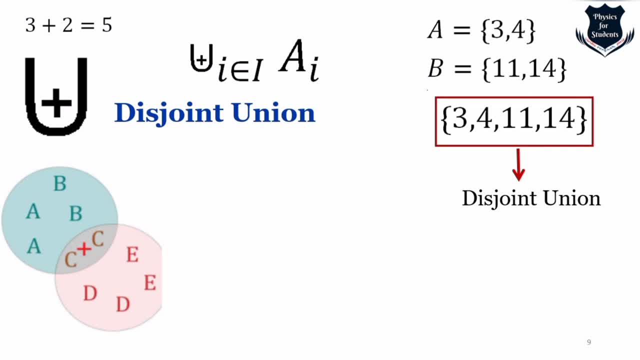 for example, these are the elements of A and B, C, D, E. Then what we do is that we do a multi-set union. That means we are adding both to A's two of B's, C, followed by the union and a plus sign. 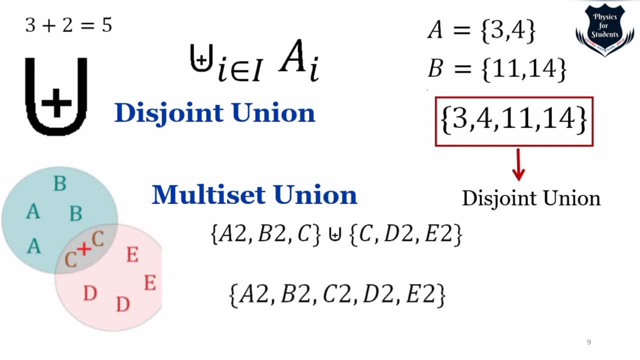 and C and two of D and E, two of which results into this Av2: B2.. c 2, d 2 and e 2, right, so we are doing a multi-set union, we are adding up, and here also the plus sign. 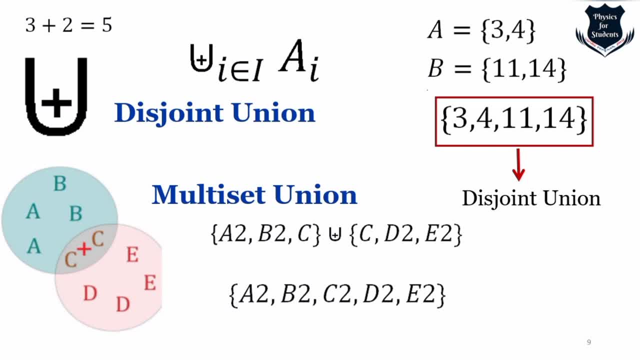 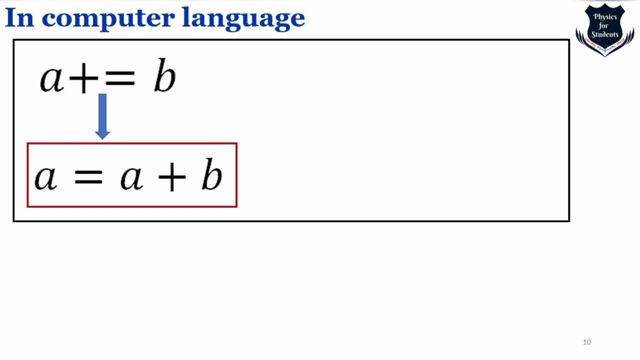 is being used inside a big u in computer language. this is used plus sign is used. a plus equals to b, which means a equal to a plus b and a equal to plus b, which means a equals to b. and if i use a plus plus, it means a postfix increment, which means returning the value before incrementing. 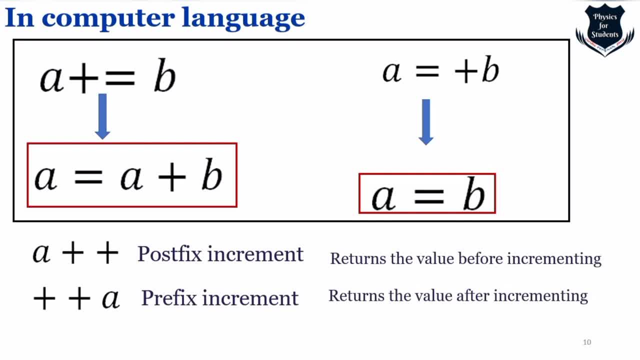 and plus plus a, which means prefix increment, that means returning the value after incrementing. so more or less this is clear, that this plus plus signifies before and plus after and this is before. so it is the value before incrementing and minus incrementing. and the computer language i. 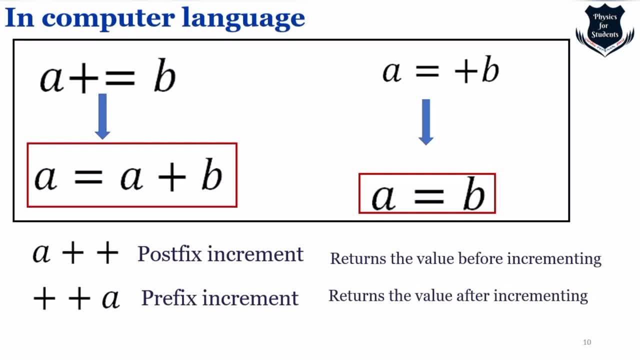 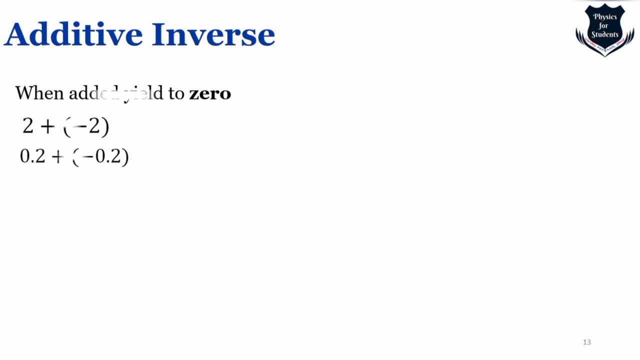 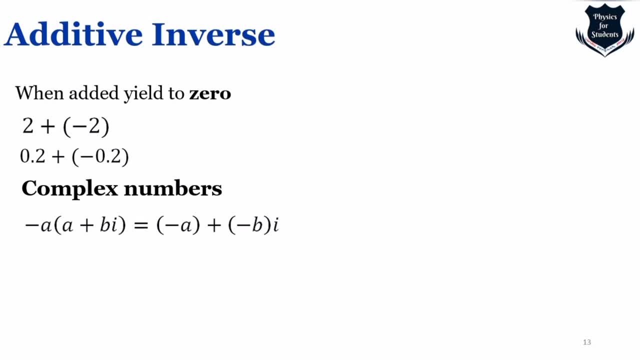 wonderful thing that once we use this in complex numbers- minus a plus B, this- and we try to plot it on a complex plane, it gives a totally, a kind of a 365 degree, a different kind of a curvature or just different kind of a figure in the 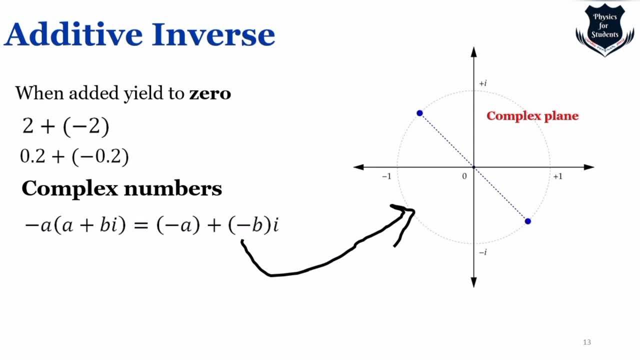 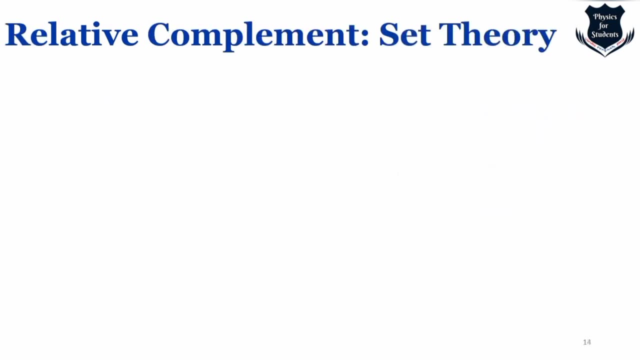 complex plane. so this shows that how we can use the additive inverse or the usage of the plus sign in a complex plane, or complex numbers, which gives a different kind of a complex plane. well, something we come across which is called a relative complement in set theory. now let me just tell you what is this? that 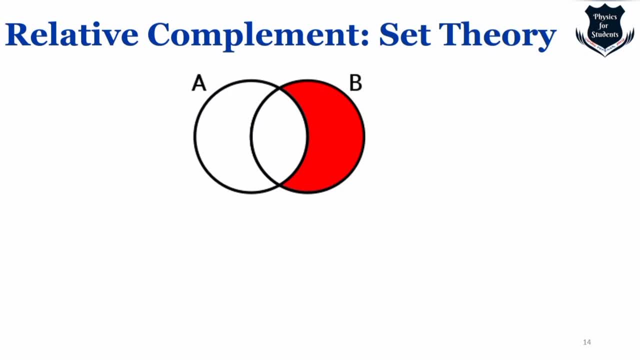 if A and B, for example, are different sets, then the relative complement of a in B is also termed as a set difference of b and a. so we get b minus a is the set elements, but hold on hold on the relative complement of a in b is. this one is a little bit ambiguous, so if you find this term, 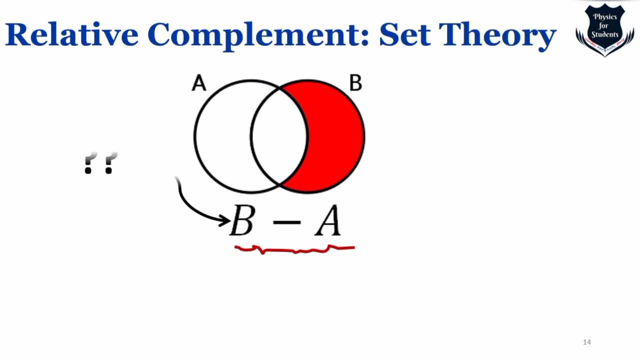 think twice whether you should consider to be right or not, because this leads to yes, the question mark. however, the right symbol is this: one right with a slash right. so this, this is something you need to be very careful. so the relative component of a in b is denoted by the green sign which i have. 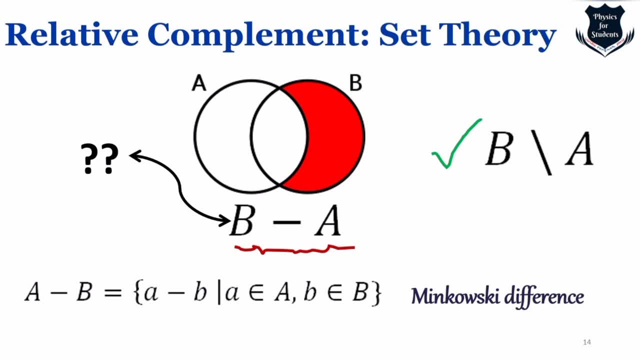 shown with a tick right is sometimes written with an ambiguous term which i have already shown, as in some context it can be interpreted as a set of all elements, b minus a, where b is taken from. where b is taken from, i mean just a small b is taken from capital b and small a is taken from. 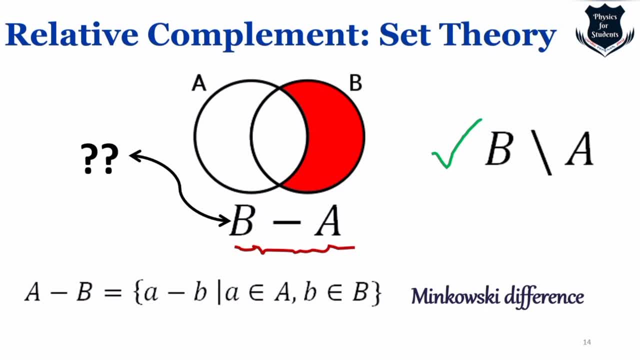 capital a. you need to be very careful. so the relative component of a in b is denoted by the green sign. there is also something at the bottom of your screen which is called a minkowski difference. however, i'm not going to go ahead and explain much on this particular subject, but just note that 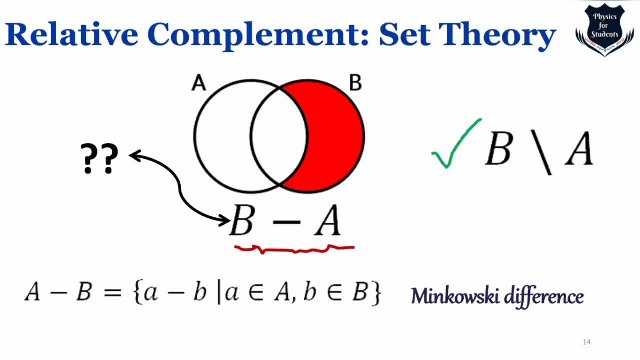 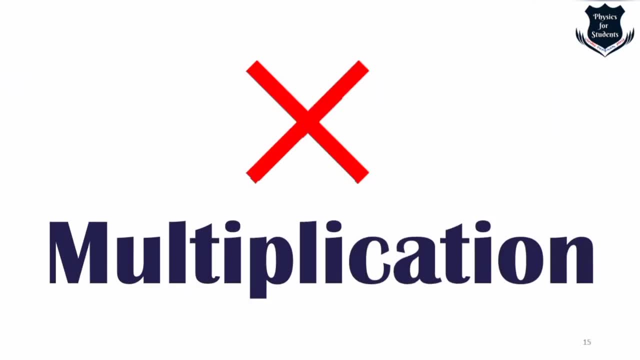 minus sign is also being used in complement set theory, which can be ambiguous, but it is very much used in minkowski difference. we come across the next symbol in arithmetic, which is called multiplication. now, multiplication has got a wonderful history which i would like to tell you. 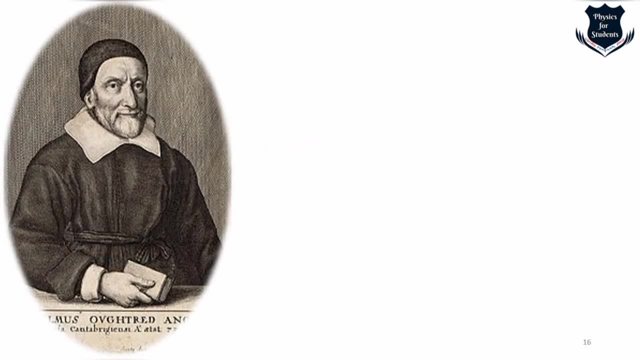 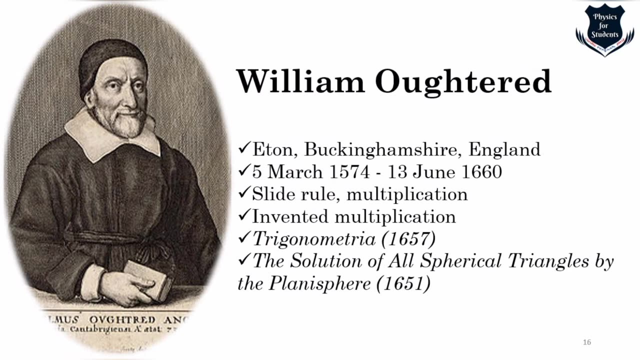 now here is a person you know is born in the year 1574, named as william outend, an english mathematician who is best known for his invention of an early form of the slide rule, which is used in algorithm, and he invented many new symbols, including the multiplication x symbol and the 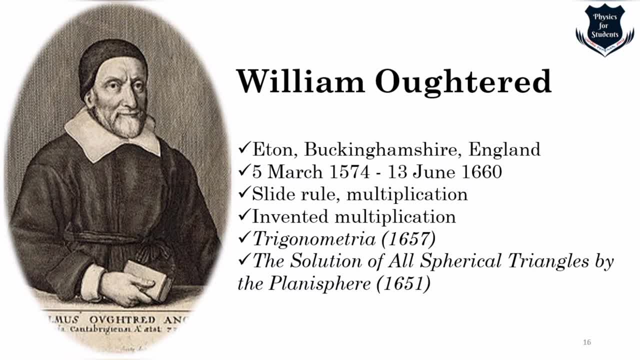 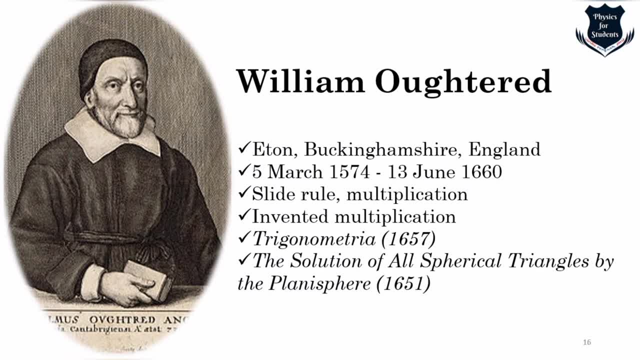 some of the biographies gives this date as his date of birth, but in fact is the date when he was baptized, so his actual date of birth is known, but is unlikely to be more than a few days before his date of baptism. william attended eton school as a king scholar which, although a very 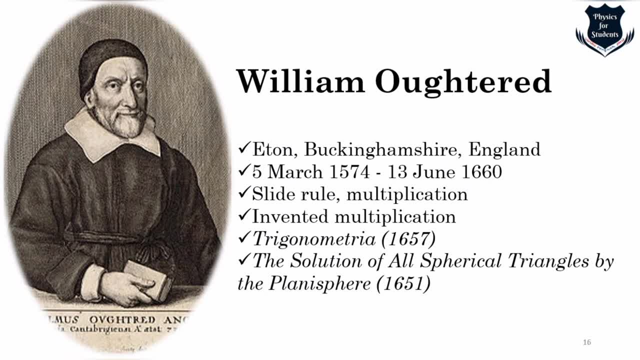 famous school was in fact his local school, the school where his father taught. william was taught arithmetic at eton by his own father. william outrend's most important work is clavis mathematica, the key to mathematics, which was published in 1631. this is a textbooks on elementary algebra. 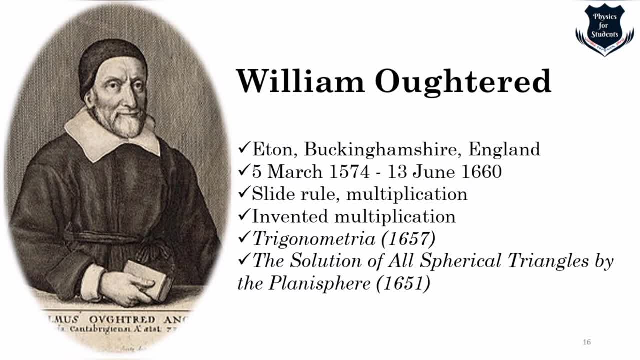 he experimented with many new symbols, including multiplication and proportion. outrend also invented freely with symbols introducing not only the multiplication sign, which is now used universally, but also the proportional sign, which is the double colon, and this book became popular around 15 years later as mathematics took a greater role in higher education. given this background of william, 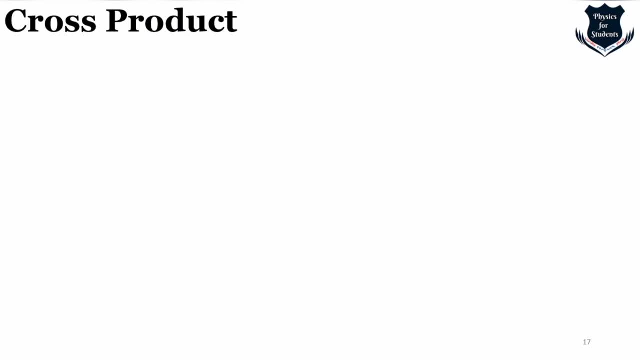 outrend. let us see that. what are the other usage of this cross multiplication sign? so across product? first of all, it is a binary operation on two vectors in three dimensional space. it results in a vector that is perpendicular to both the vectors. now you see this: a and b. once i put across product it looks like this: and if a and b multiplied produces another. 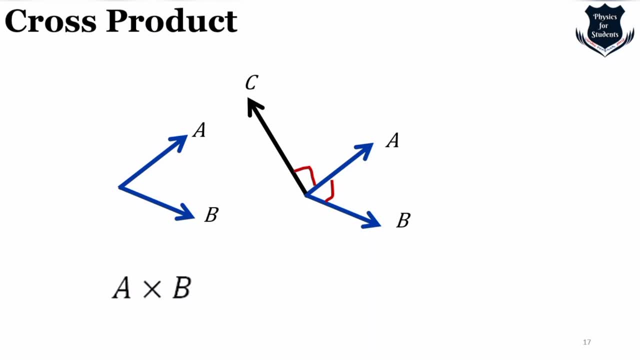 vector c, which should be perpendicular to each other- and i have shown it in black so that you can understand- and it is the value, should be sine theta. so there are other various notations, i would say various implications and detailed understanding of a cross product, but that is beyond the scope of this video. 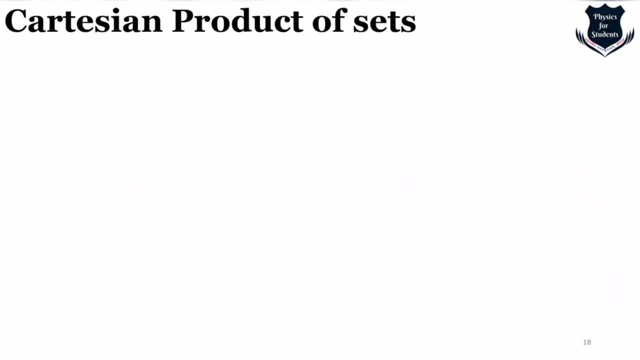 we also say what is called the cartesian product of sets. where i have just taken abrupt, a is equals to egg and chicken and b is a set of sausage and chips. and when you do a cartesian product you get egg, sausage, egg and chips and chicken and sausage and chicken and chips. 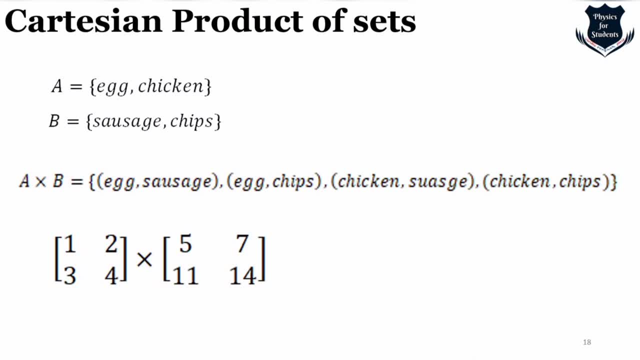 so what we get is something like this. so it is typically a cartesian product of sets. you see, the multiplication sign between the two matrices now hold on. you might also ask me that why this multiplication sign? can there not be a dot sign? yes, definitely. later on in linear algebra we get a dot sign. but in case of elementary linear, 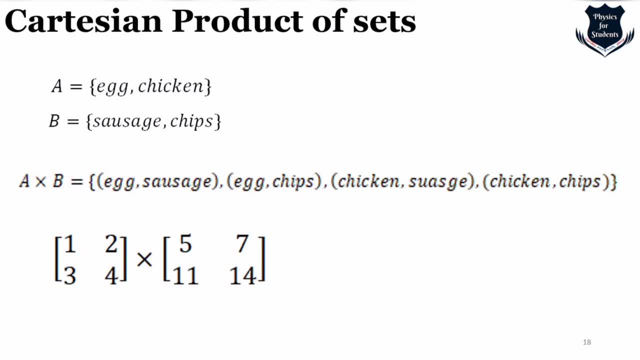 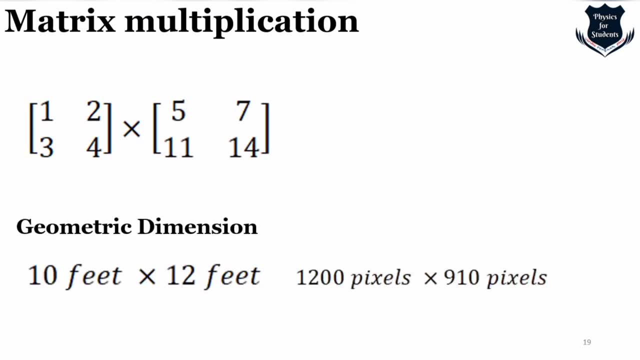 algebra, in matrix multiplication we use this sign, so it is worth mentioning it is also used in matrix multiplication like this: and it is used in geometric dimension, for example, 10 by 10 fit house or a room, or to mention the resolution of the computer screen or a laptop screen audio. 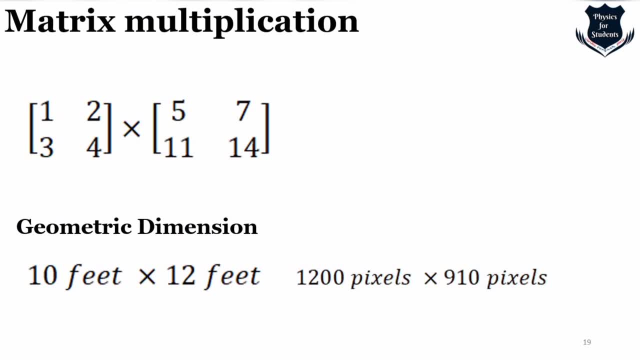 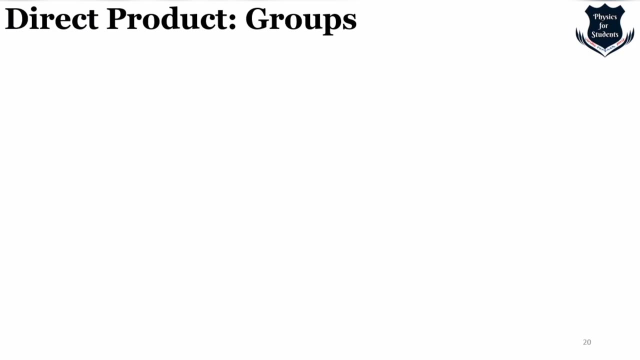 television we use 1200 pixels by 900 pixels, or 20 pixels by 50 pixels, and so in all it, it mentions what is called a geometric dimension. now, here is something very interesting: what is called a direct product of groups. now, hold on, i'll just like to mention in a few words, so that 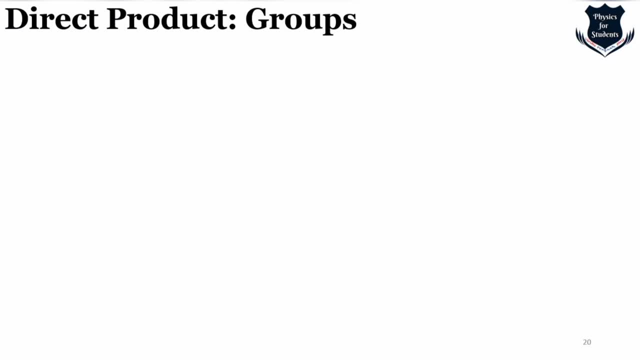 you can really enjoy the beauty behind that now in mathematics, what happens specifically in group theory? the direct product is an operation of two groups. so just for the time being, let us not go into the details of group theory. let us understand: there are two groups, g and h, which constructs a. 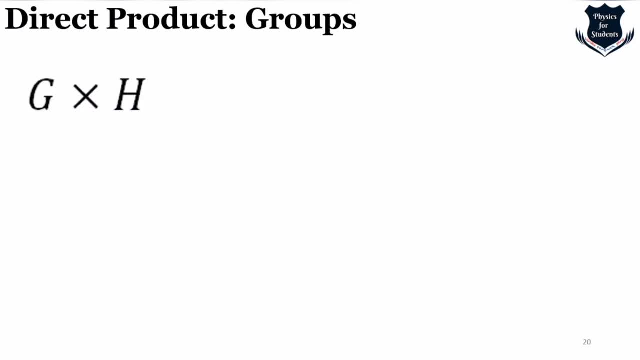 new group denoted by this right g multiplied by s. this operation is somehow a group theory. the direct product of group theory is actually an operation of the Cartesian product of sets and it is one of the several important notions of direct product in mathematics. now the direct product is defined for a number of classes. so you see, this is the direct product. 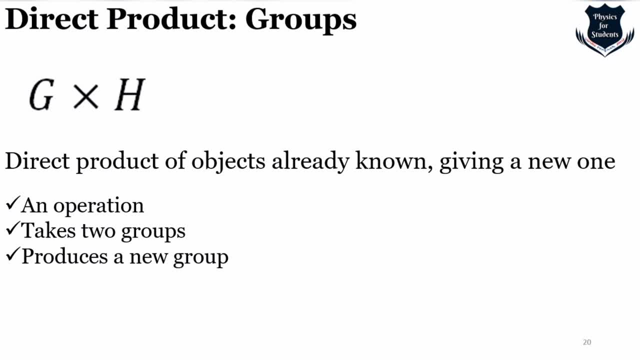 of objects already known, producing a new one. it is an operation, it takes two groups and produces a new group, right. so in case, in each case, the direct product of an, of an algebraic object is of its elements, consider its sets- and its algebraic operations are defined component wise. 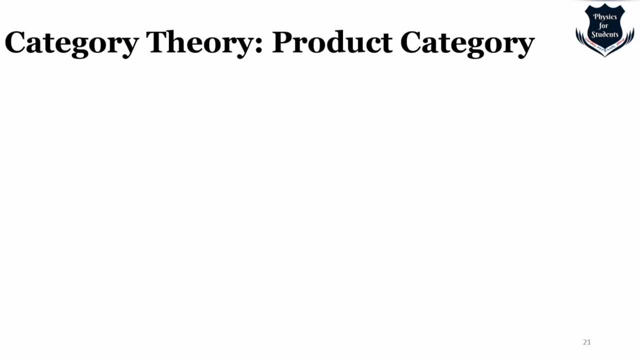 so direct product is another important where the multiplication and is used. another important is using it in category theory, producing a product category. just a few lines, you will be able to understand what is category. now. a category actually describes the essence of objects, right. so category theory assumes that we can determine essence by knowing the 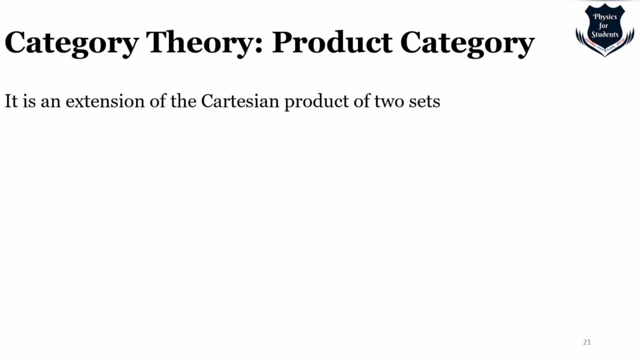 relationship among objects. so I want to emphasize: so it is an extension of the Cartesian product of two sets. so what I want to emphasize? that we don't actually care about the nature of the objects themselves, we only care about relationships. so objects matter so little in category theory that we often just call them things. however, we give all sorts of 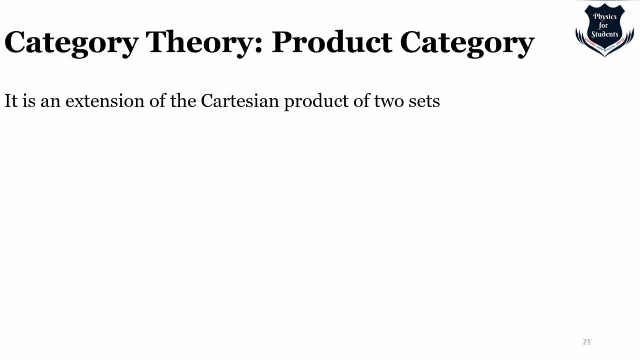 names to the relationships, something likes monads, monoids and groupoids, and so on. so the general guiding principle in category theory, though, is: what is important is not what an object is right. it is not important what an object is, but rather what it does, how it behaves relative to other. 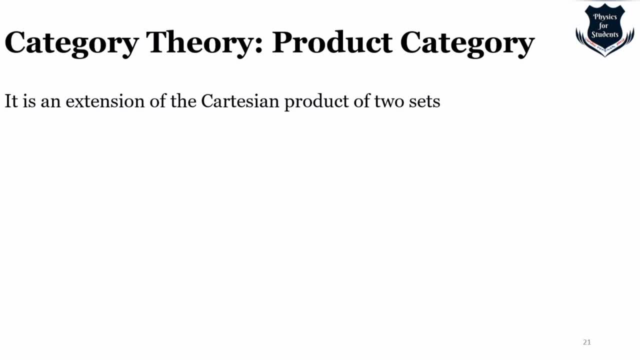 objects in terms of morphism. so these words describe different kinds of categories if you think of them as different classifications of relationships between things. so in mathematics, a field of category theory, we take two categories, c and d, denoted by this, and it, product of two categories c and d, is denoted by, so on. so this is another important usage of multiplication sign. 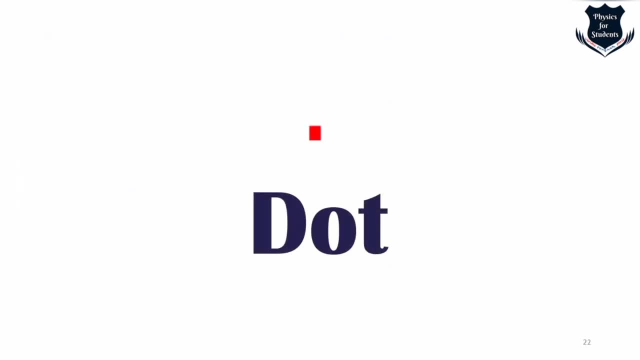 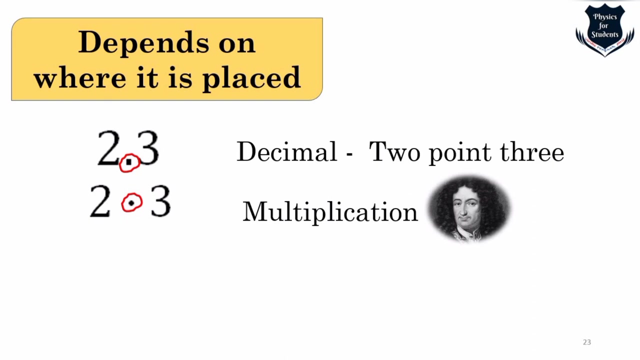 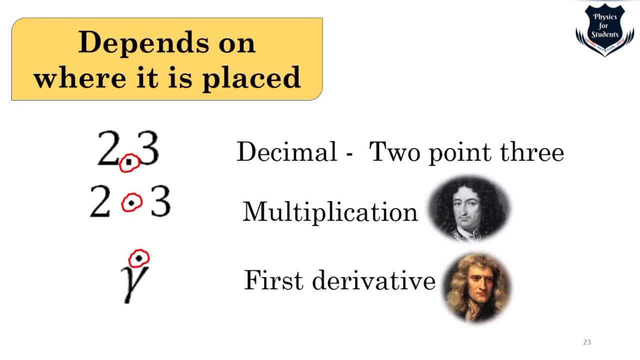 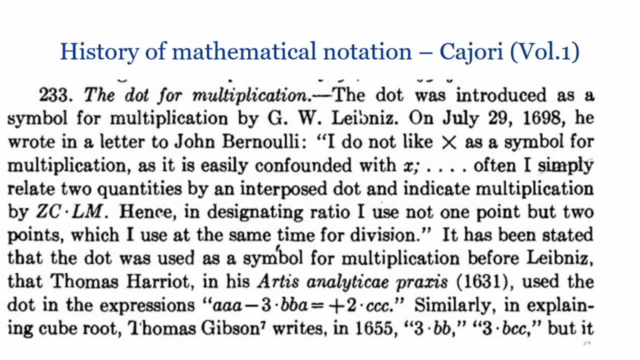 on the point. depending upon the position of the point, the meaning of the dot changes. now here is a note, again from kajuri's book, very important and interesting, that leibniz, on july 29, 1698, wrote a letter to johan bernoulli, another great mathematician, that i do not like the cross as a. 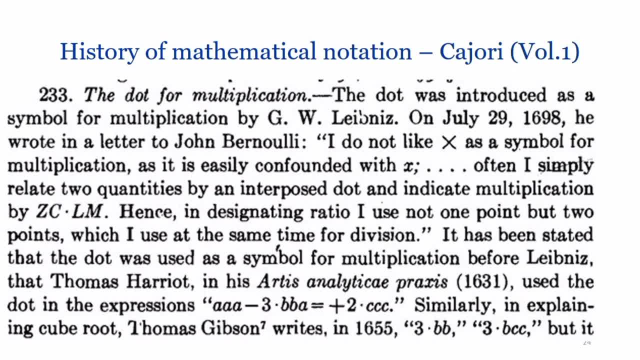 symbol for multiplication, as it is easily confounded with x. that means it gets complicated often. i simply relate two quantities by an interposed dot and indicate multiplication by this one. if you read further to this paragraph, you will sign that it has been stated that the dot was used as a symbol for multiplication before leibniz. 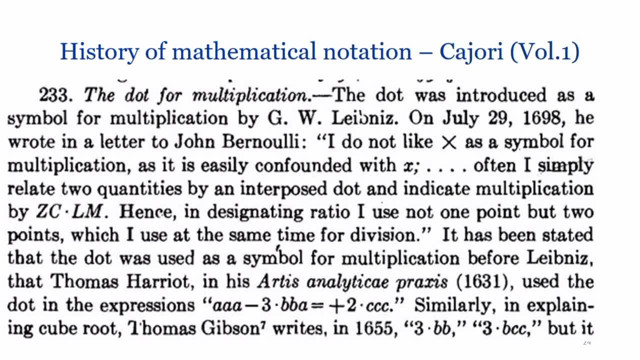 that thomas harriet, in his this book, used the dot in the expression so on. so this is just an interesting historical. uh, note that how leibniz wrote to bernoulli mentioning that he is going to use the dot as a symbol for multiplication and that he is going to use the dot as a symbol. 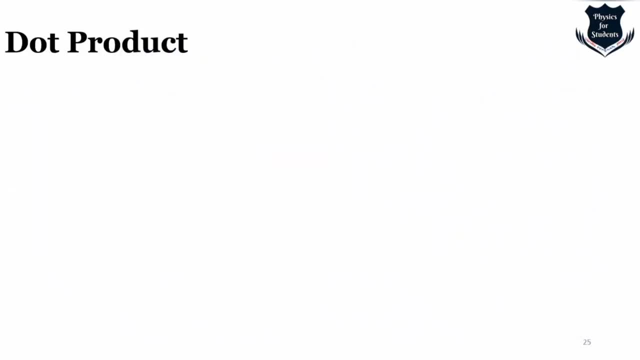 for multiplication- and that is why he is getting confused- using the cross and instead of that he used a dot sign. now this dot is also used to denote what is called a dot product. i'm not going to define or go further details in what is a dot product, but algebraically the dot product is: 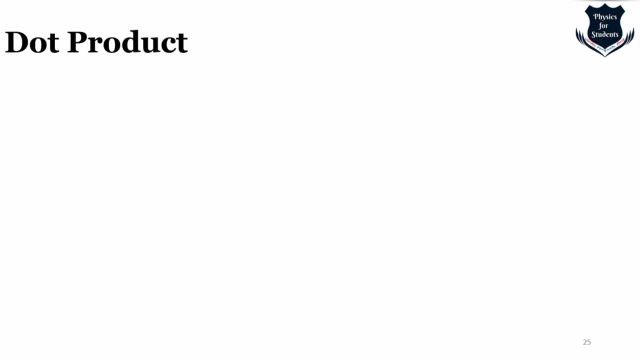 defined as the sum of the products of the corresponding entries of two sequence of numbers of euclidean magnitudes and the cosine of the angle between them. so both the definitions are equivalent. when working with cartesian coordinates, however, the dot product of two vectors is the product of the magnitude of the two vectors and the course of the angle between them. 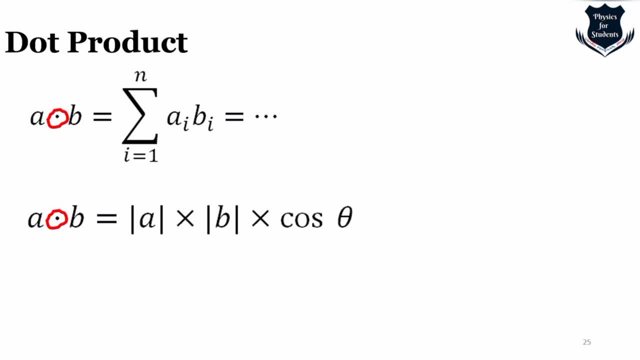 in mathematics, the dot product or scalar product, is an algebraic operation that takes two equal length sequence of numbers and returns a single number. so right on your screen i have given two notations of dot product. i've used a circle marked in red so that you can understand that. 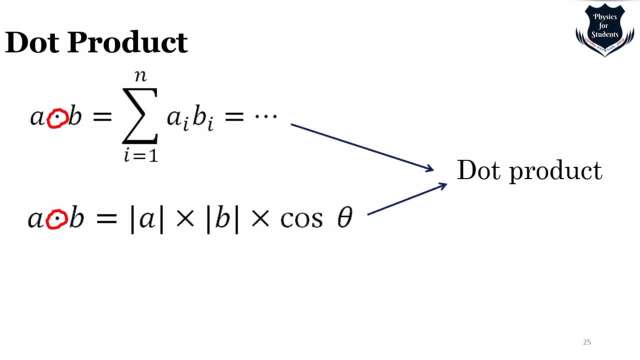 the usage of the dot sign in terms of dot product. both of these means dot product. now here is a note of attention: often on you will see that the dot product, which is just a single dot, can be get you get confused with this one. now this is not a dot product, if you are aware. 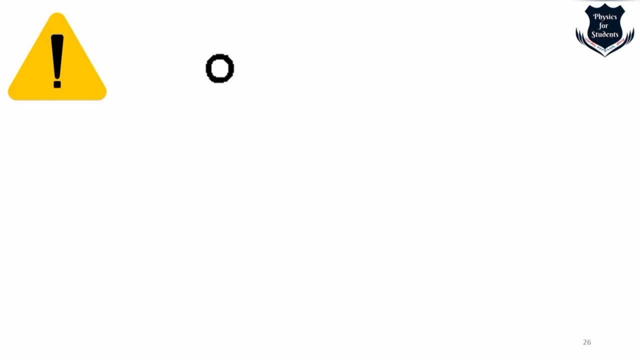 about using microsoft word and using the dot product. this is correct if you are a major после the symbols in microsoft dot or you're using latex symbol, this is different. this is called a composite function, to be- to be on simple words, a function that is written within another function. 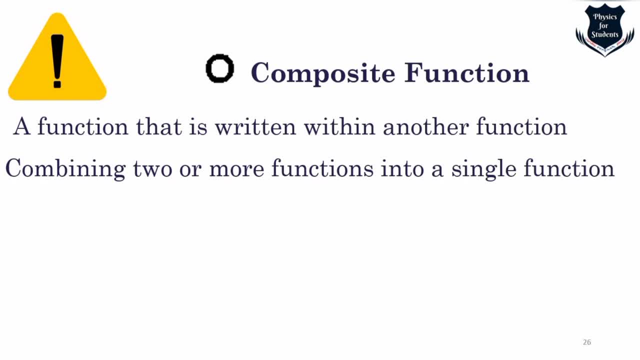 is called a composite function, so that dot, which is just a single dot, a point- uh, adjust, just a small one is, should not be confused with the composite function. let me give you a very quick and a simple example how to understand a composite function. so let us assume that x is the flower we 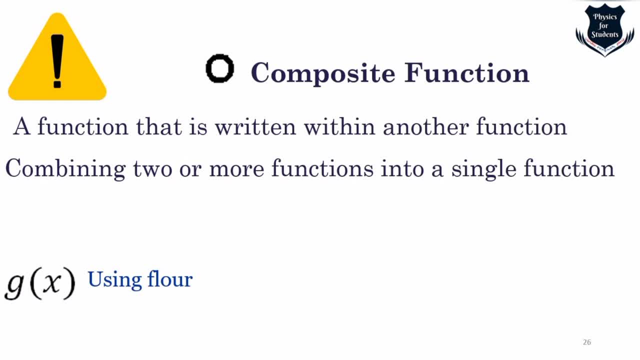 are making bread. right, it's nice winter season still here, so we are making bread. so let x is the flower, the food processor is doing the function of preparing the dow, of you know, making the flower, and we call it gx, and let the oven, which is f of x or x, makes the function of. 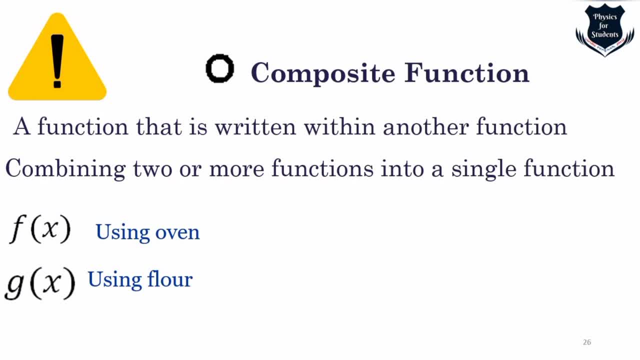 making the bread right. so in order to prepare bread, the output is this one right. so g of x should be placed in the function of f of x. that means what? that it the, the prepared dow should be placed in the oven. the result is denoted by this and i have marked this in red. so 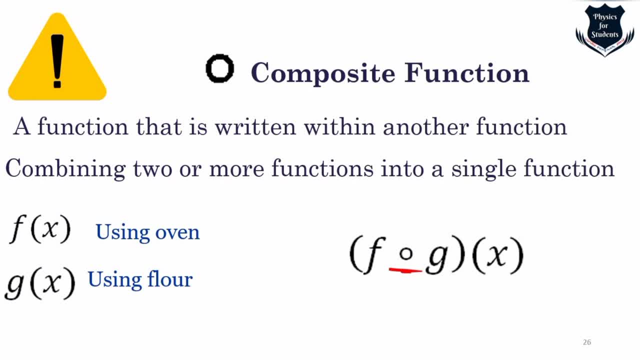 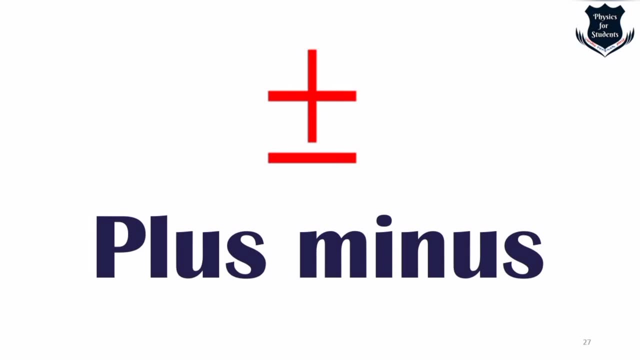 that you understand that this is a composite functions of g, of x, using flower, getting processed into oven and producing the final result through a composite function which is a nice tasty bread. so we come to the next part of arithmetic operator, which is very common, which is called a. 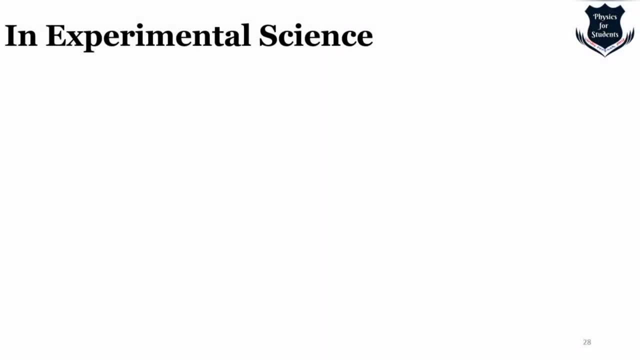 plus minus. now, in experimental science, we all know that 40 plus minus 5 actually means the range should be between 35 and 45. right you know it is. it's quite simple. so it defines the range and the margin of error. and if we take a ruler and we mark something like this, so it 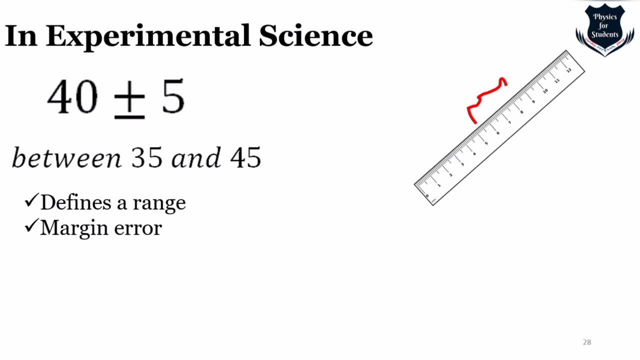 means that the margin of error should be between, say, 5.5 and 8.5, right? so we sh show a figure on the right hand side of your screen and this is the value. so the value could be between six and a half and seven and a half, right? so this is plus minus 0.5. so we say that. 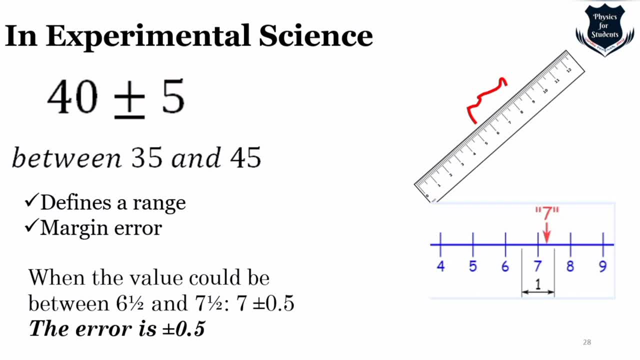 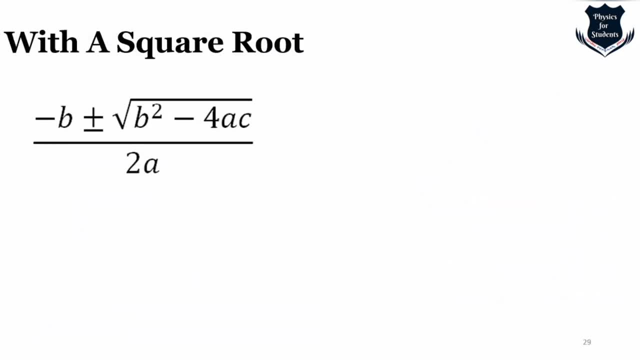 the error margin can be something between plus minus 0.5. so this is the usage of plus minus in experimental science. now we all know that if we get a square root or a quadratic equation, it means that we will use both the positive and the negative sign in order to get the result of that. 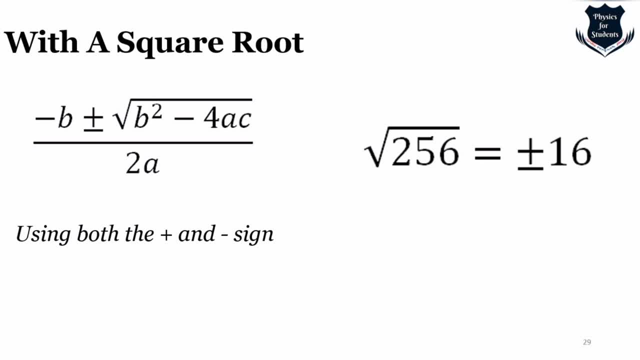 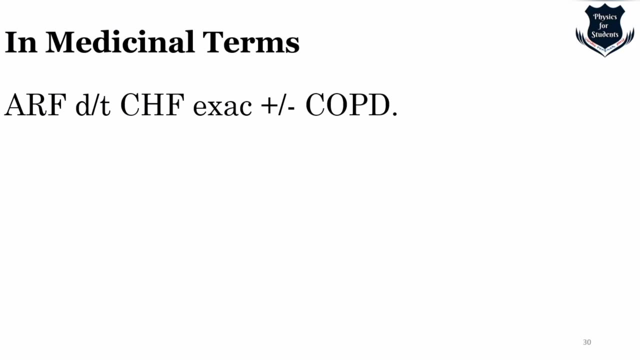 equation. so square root of 256 means we get a positive 16 and we get a negative 16. so that is the usage of a square root. this is something very interesting. now, in medicinal terms, the doctor usage this word right. it is not a very good thing, but anyway, just as an as an. 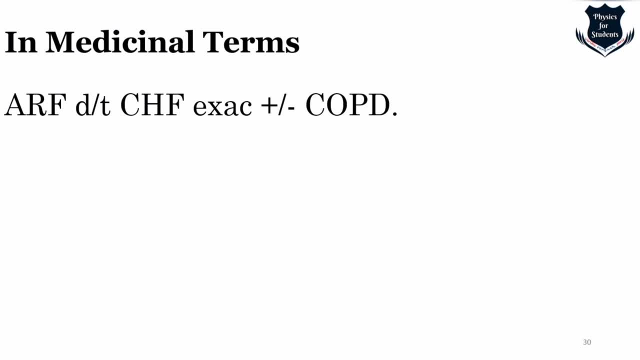 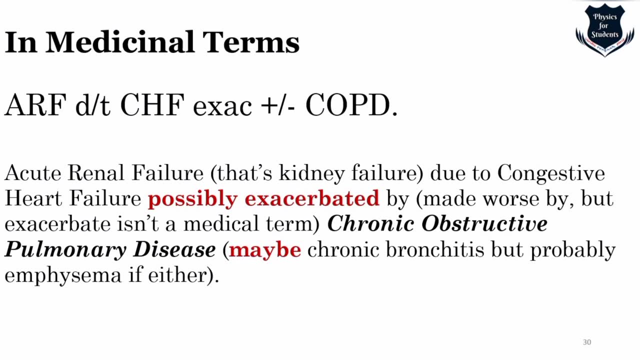 citing as an example. so in medicinal terms, if you use this, what does it mean? if i translate it, it says acute renal failure. that means a kidney failure due to congestive heart failure, possibly excavated or made worse by the excavate isn't a medical term. 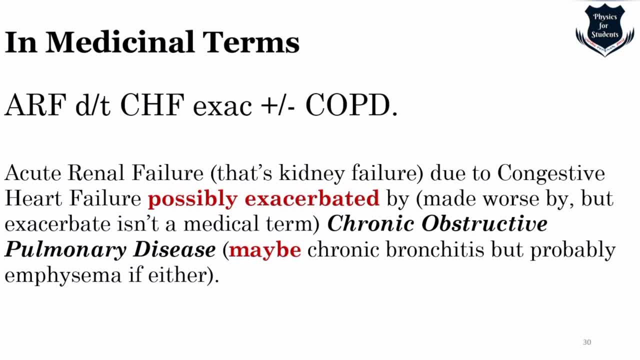 chronic obstructive pulmonary disease may be chronic bronchitis, but probably ephesema. if either so, what i am trying to tell you is that if you see that the doctor is using the plus- minus sign in medicinal terms, it means that it is more or less this or it is coming close. 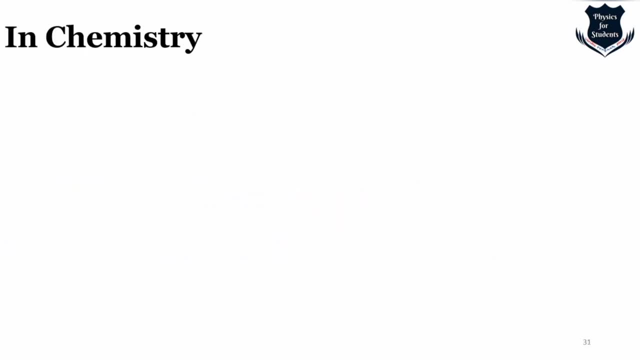 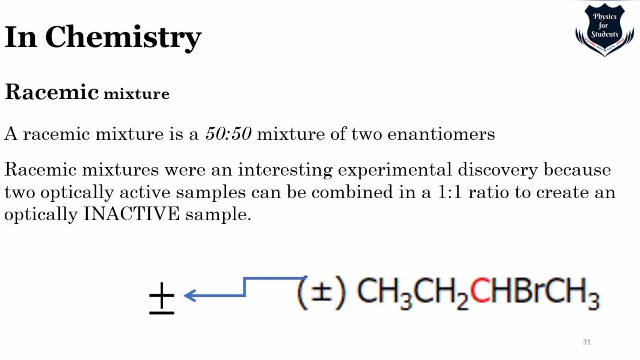 to that. now in chemistry it is used. this plus minus science is also used. now here is a new uh. it is something very new for me. it is called. this is a term which is called a russimuk mixture. it is a 50 fixedly mixture of uh of two another in a. this is called an enatimus right, the enatimus or arrays. 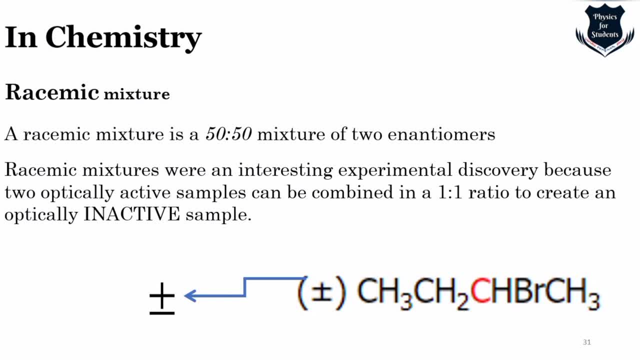 the russimuk mixtures were an interesting experimental discovery. between two optically active samples which can be combined in a one is to one ratio to create an optically inactive sample. so i'm not going to be very honest. i'm not the right person to tell about russimuk mixture, but here 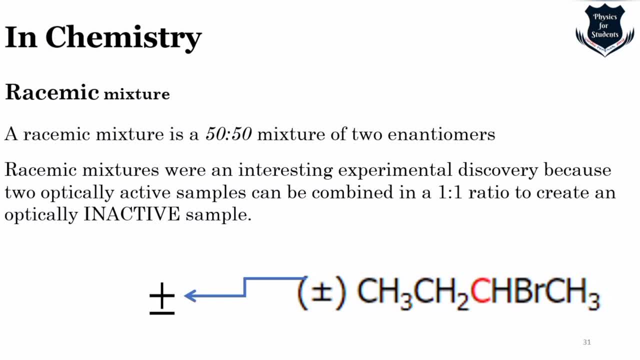 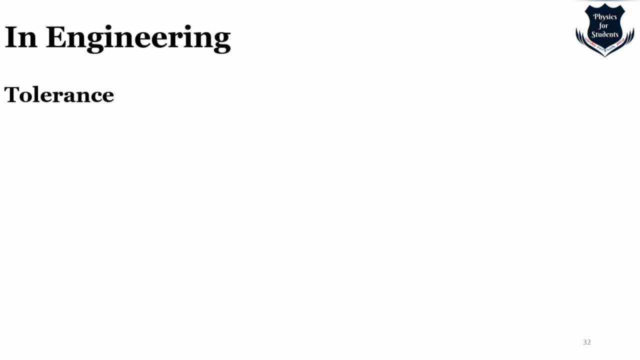 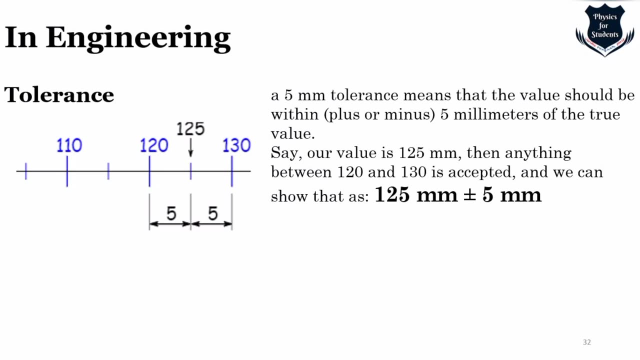 is the plus minus sign used in chemistry. so just to give you an idea, in engineering, if we go forward and we understand, there is a concept called tolerance, which also says: say, for example, this kind of a figure on your left hand side. so what does that mean? it means a five millimeter tolerance. 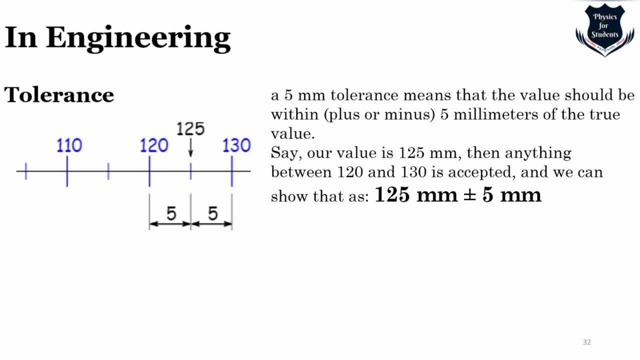 the value should be plus or minus five millimeters. so our value, 125 millimeter, has any range between 125 and 30 and we say 125 mm plus minus 5 mm. so the concept of tolerance means the range of values in which a measurement is acceptable. so it can be anything. it can be measurement problems, it can be. 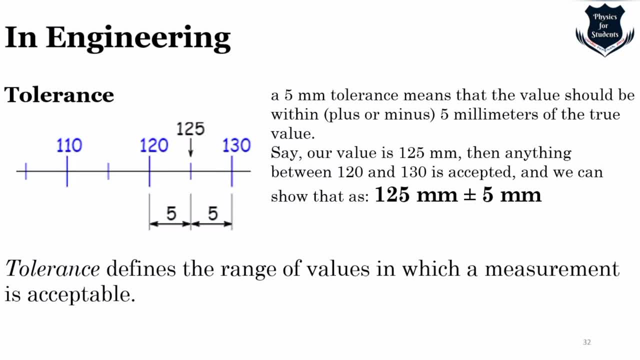 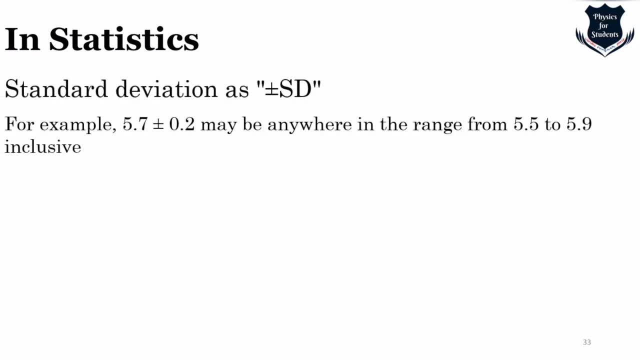 anything which will come more clearer in the next, in next few seconds. so engineering tolerance is this? now, in statistics, for probability and standard deviation, we use this plus minus sign, right. so plus minus, 5.7. plus minus means it can be anything between 5.5 and 2, 5.5 to 5.9, inclusive of that. now here is the concept which 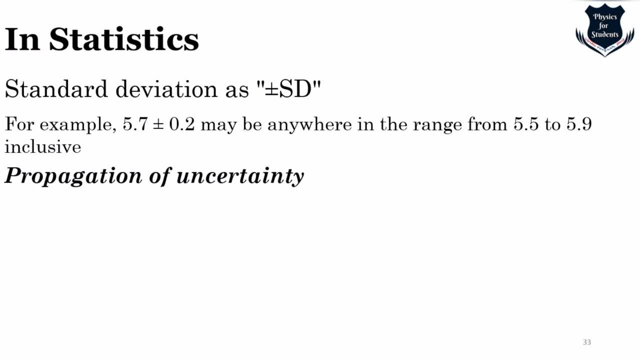 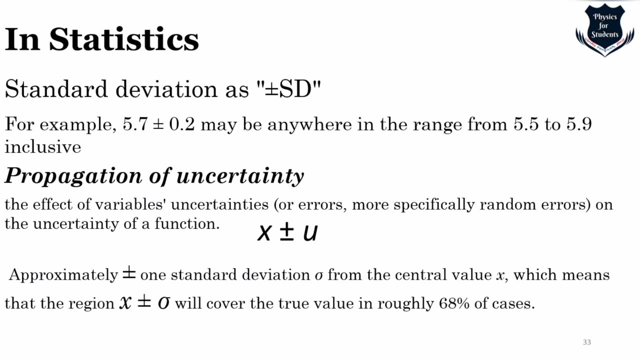 is called propagation of uncertainty. now, in statistics, propagation of uncertainty is the effect of variables or uncertainties, i would say on the uncertainty of a function based on them. now, when the variables are the values of experimental measurements- right, we are experimenting something- they have uncertainties due to lot of reasons. temperature, air pressure measurement limitations instrument. 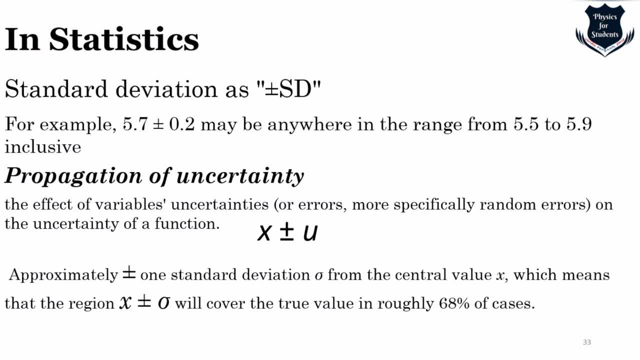 precision and this which propagates due to combination of variables in the function. this is what we call propagation of uncertainty. so you see the effect of variables uncertains on the uncertainty function. x is plus, minus, mu or whatever. so approximately you can see that here, for one figure, we have one evaluation signal song. so for example of ru, 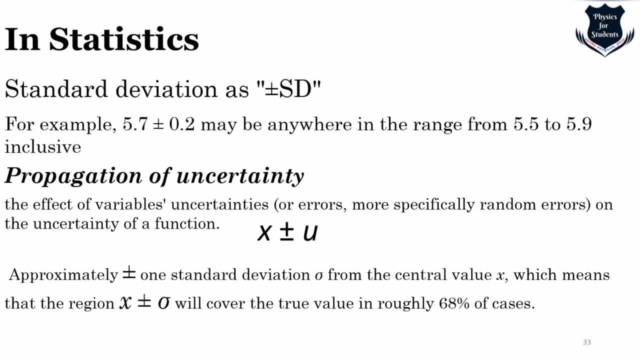 this question. I have started this commonry and it is showing thearte of the mij for 1. this is isn't as bad, but we are at big round bar, yes. the other major problem, which is the there are no aquiloians and one is 거미우, and this is zero order- one be000- and then another. there is going to be square wyca bookstore. even today you may see one standard deviation from sigma, from the central value. it is roughly around this case. so in standard deviation as well as in propagation, you will see more in quantum mechanics, when we use this, that there is the uncertainty principle: plus minus due to several external, extraneous factorsrer� 안돼 adjust factors. so there is another one which is: 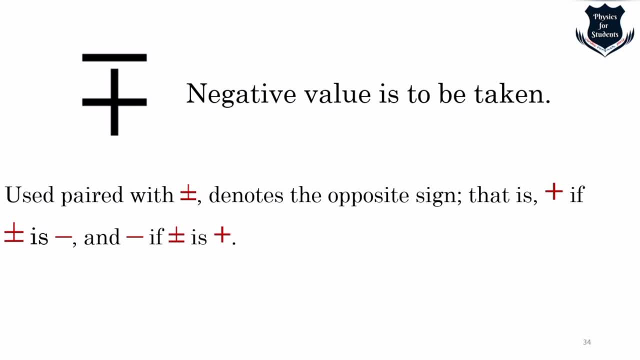 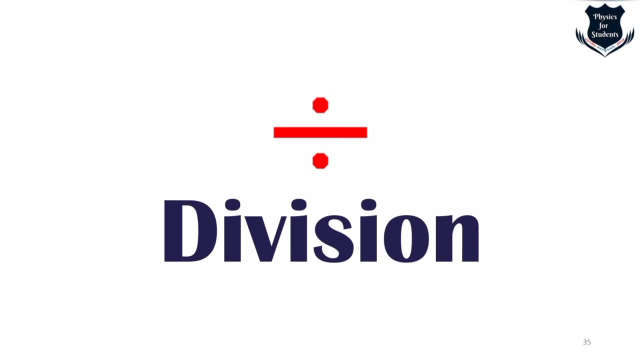 plus, so it means that the negative value is to be taken. I have written that used pair with plus minus denotes the opposite sign. that means if there is a plus, if plus minus, we take the negative and minus, if plus minus, then we take the positive. so we come to another interesting arithmetic operator, which is: 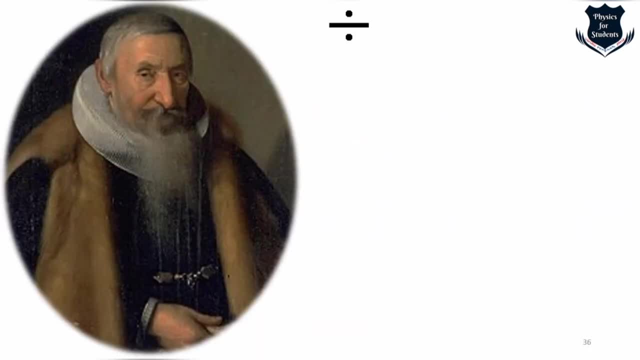 called the division. now this has got a very interesting. you know history. now this word I will explain to you, the person who is shown on the left, this word, the word obelisk, actually comes from the Greek word obelos, for sharpened it means stick or split, or pointed right. so this has the same root as you. 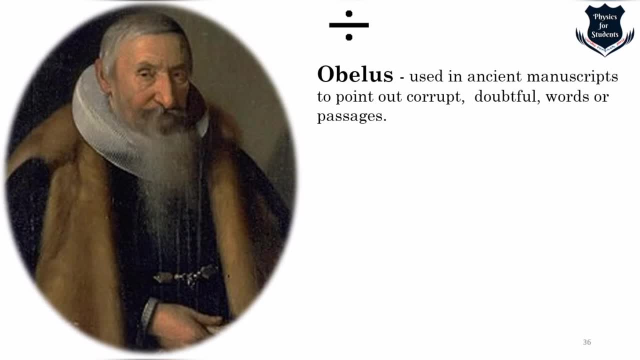 understand of the word obelisk, which means you know Church, we see obelisk right. so the form of the obelisk as a horizontal line with a dot above and a dot below, and was first used as a symbol for division by this Swiss mathematician. 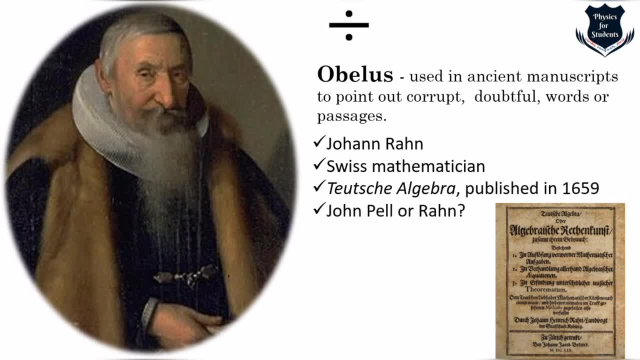 Johan Rahn in his book touch algebra, which was published in 1659. right at your bottom, I've given a small picture of this book, and this gave rise to the map, modern mathematical symbol. Johan Rahn was actually was a Swiss mathematician who is credited with. 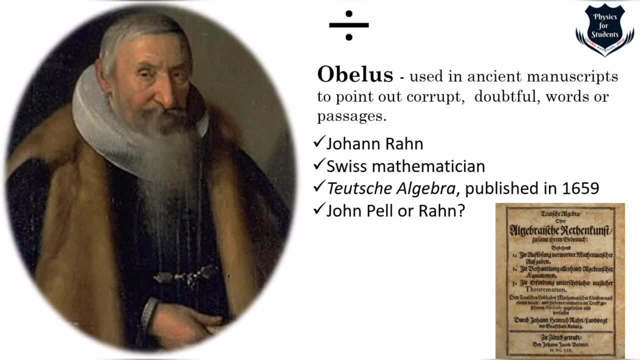 the first use of the division sign pre. it is supposed to be a obelisk variant and therefore a sign and a therefore sign the symbols used in touch algebra, published in 1659. another mathematician, John Pell, collaborated with Rahn in this book, which contains an example of the 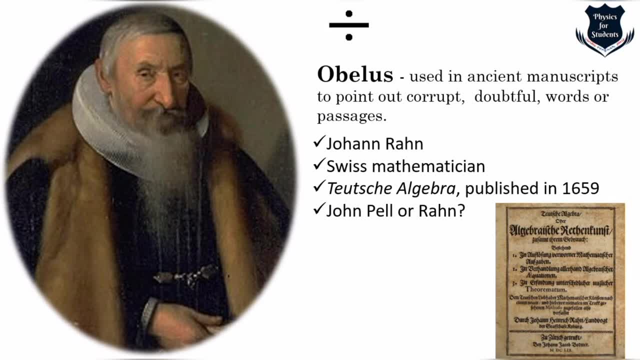 pale equation. it is uncertain whether Rahn or Pell was responsible for introducing the symbols. that means there is still- and you know, history is full of problems and full of different kinds of opinions, and in this case the obelisk sign of Rahn and Pell is also not an exception. 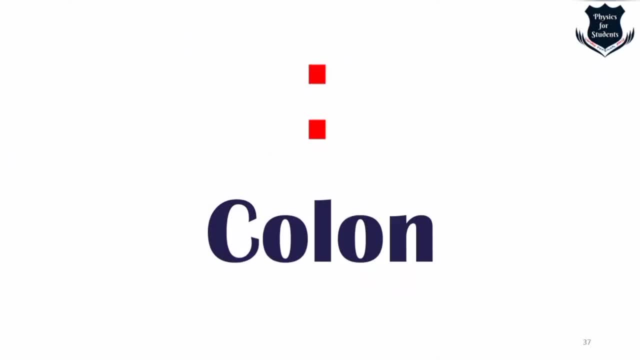 I'm not going to, you know, cover up much about division, because division sign is used mostly in case of only division. now, colon, now this is something important. this is an exception. this is not a mathematical sign, this is a punctuation Mark. that means, in due course of dialects, of talking and giving. 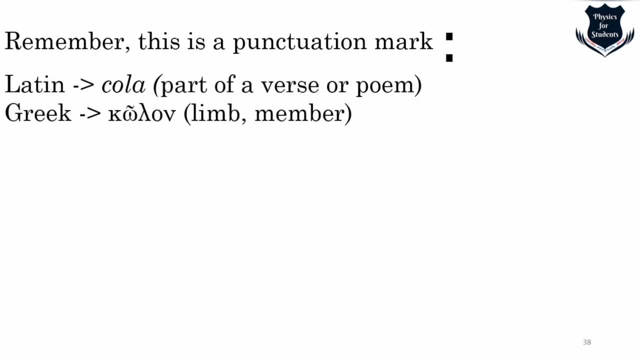 intervals. while talking this punctuation Mark colon is being used, so it comes from Latin cola, which is a verse or a poem, and Greek limber member. it has been used for various ways. few examples, so they are in front of you. I have three brothers followed by a colon. the party starts. 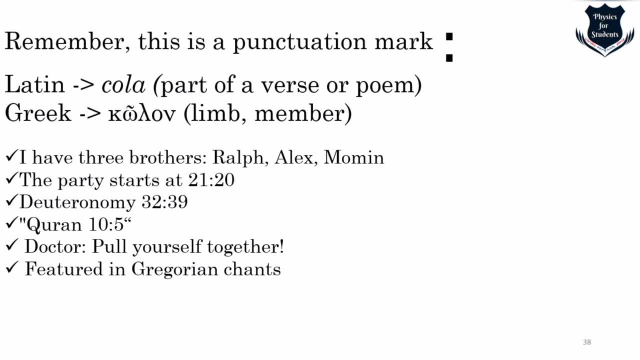 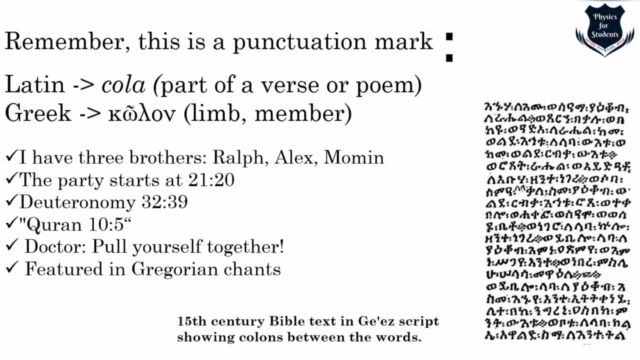 followed by a time. it is used in in Quran and in Bible, as well as in Gregorian chants. now, this is one symbol. I would say an excerpt from the 15th century Bible text, in geese, which says- and you can see vividly that the script showing colons how they are used between the words. now this: 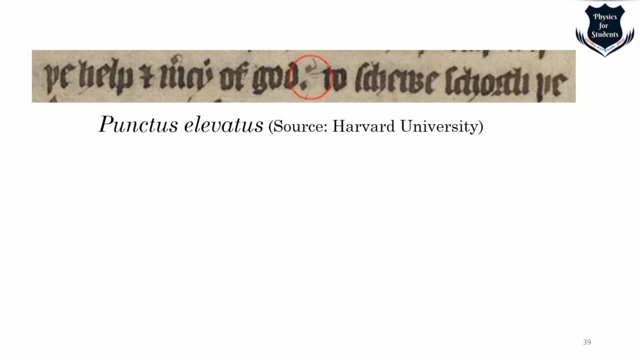 is something very interesting. now I have taken this door source from Harvard University and it means punctus elevators. now you should understand that both colon and semicolon were featured in the Gregorian chants. that means in in church or even in Operas, where the sopranos singers were there, there were usage of colon. that 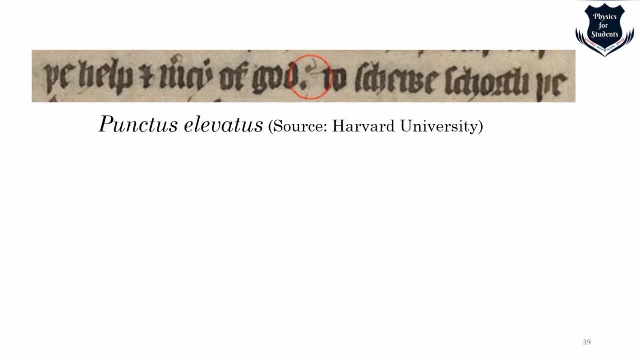 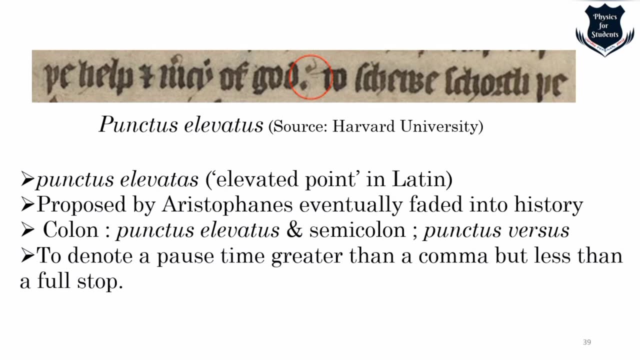 means you have to pause right, with the form as punctus elevators, which means an elevated point, colon was used as as punctus versus, which means a long pause right. it was first proposed by aristophanes and eventually faded away. so the first usage of the colon dates back to 1600s to denote a pause time. 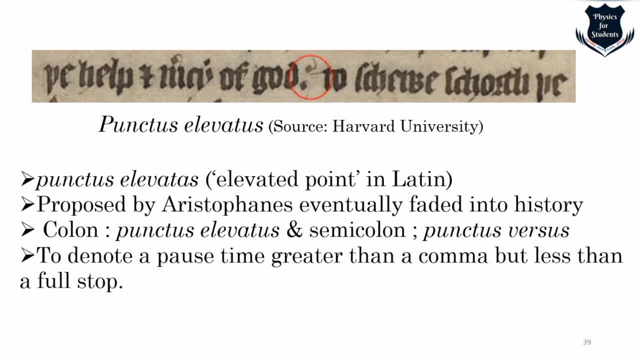 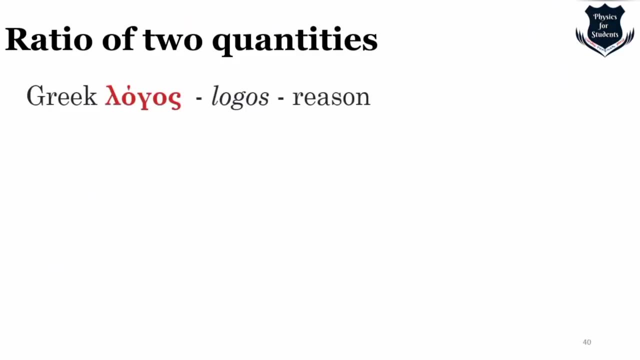 greater than comma but less than full stop. so it is a pause which is greater than comma but less than full stop. so it is a basically a punctuation sign, which later was used in mathematics is a very important point. now it is used to denote ratio of two quantities. the word ratio comes from the 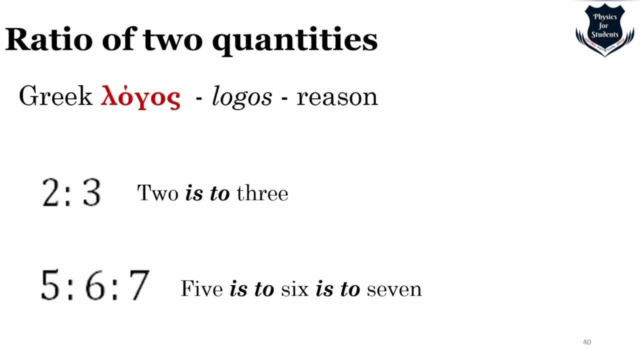 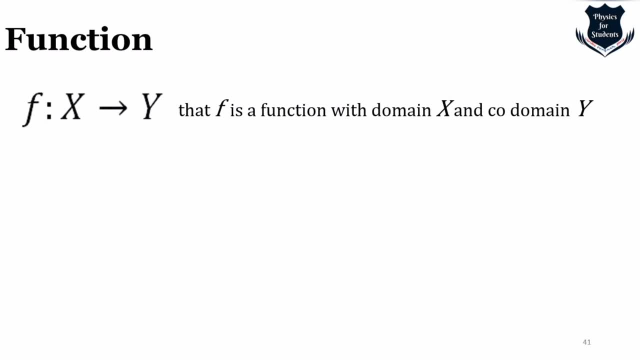 greek word logos, which means reason, is nothing great to explain. 2 is to 3 and 5 is to 6, 26 to 7. the same thing is used in colon, is used in function. so you can see a function, this one, which means a set X to a set Y, is an assignment of an element of Y to each element of X, right so? 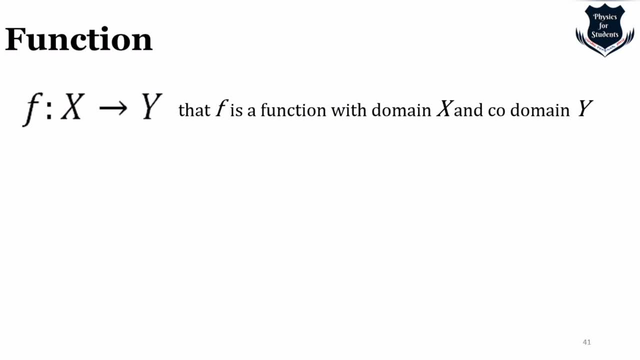 the set is called the domain of the function and Set Y is called the domain of function and in group theory it is used as an index of subgroup g, colon h, followed by two horizontal bars and the square bracket and the braces. i'm not going to explain further in group. 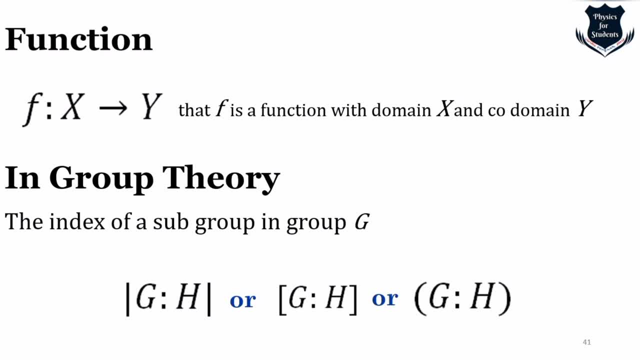 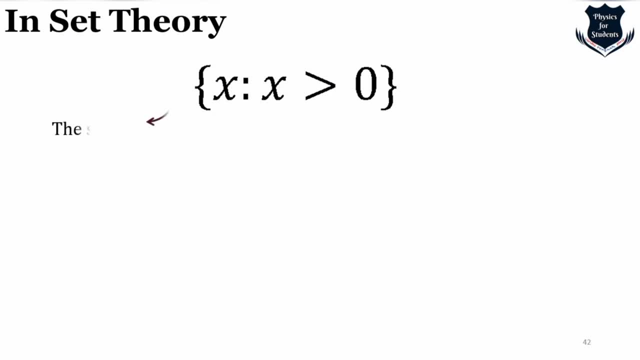 theory. but just understand that this is the colon is also used here in set theory. if you get this kind of a notation where the colon is being used, it means the set of all x, such that x is greater than zero, right? so this colon is used in what we call this kind of a notation, which is called the. 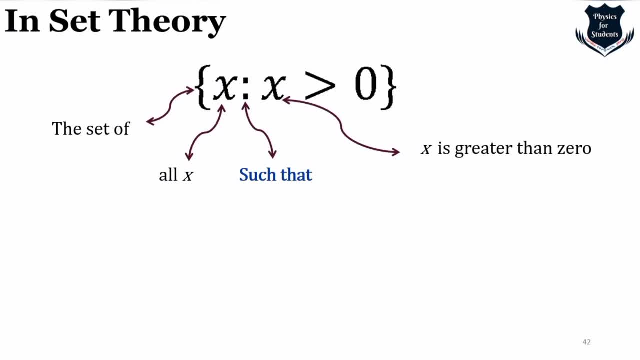 set builder notation. but remember that this colon is sometimes replaced by a piping sign, a horizontal bar. that is also means such that, and if you get this kind of an expression, it means real numbers such that, whatever the condition greater than three or less than so in set theory also colon. 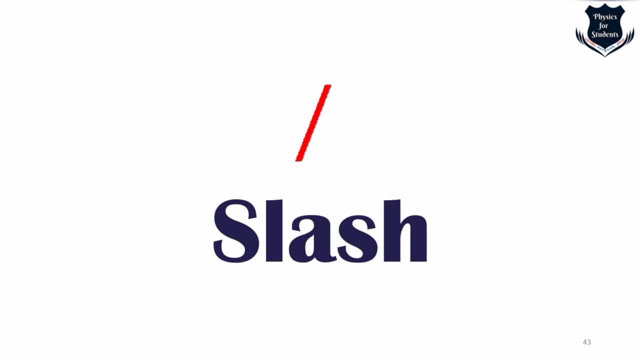 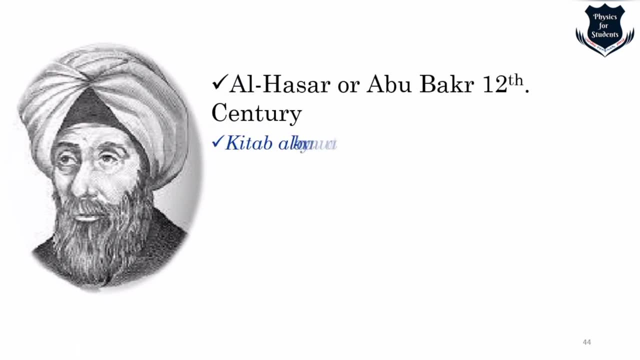 is being used slash. the origin of slash go back to a muslim method in names that. we have done a last thing and that may not have been very much of an explanation in itself. we have been introduced to taking alphabetical application to some local data encodings, and this seems all complicated, so you'll see what is kind of an American. 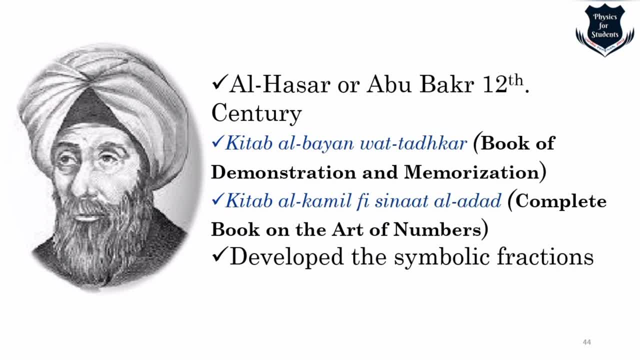 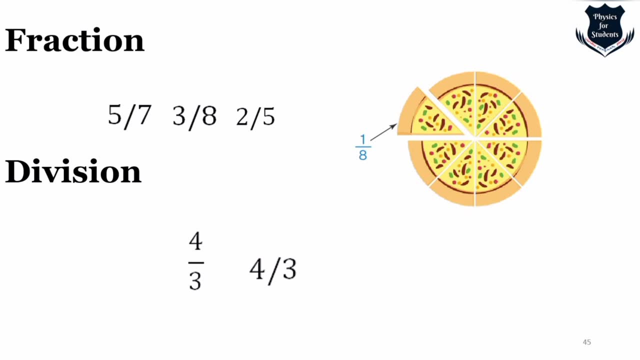 chart right on the arts of numbers. names are in arabic, so these are the two important books of al-hasr, and he is considered to be the founder of the slash sign fraction. obviously it is before you. i've just given a small pizza example to understand things easier. it is used in fraction five by seven. 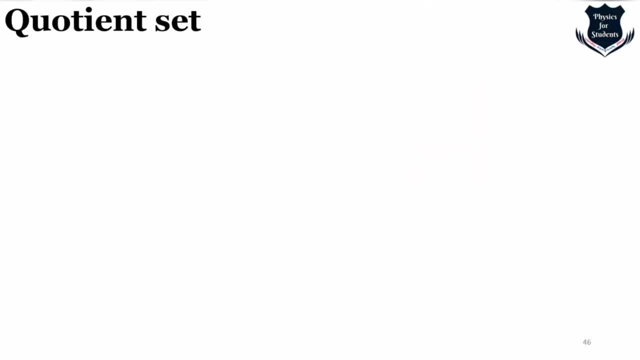 and in division also. now here is an important point. this slash sign is also used in what is called a quotient set. i will just tell you: a quotient set of a set is informally a new set obtained by identifying some elements of the original set. it is written something like this: 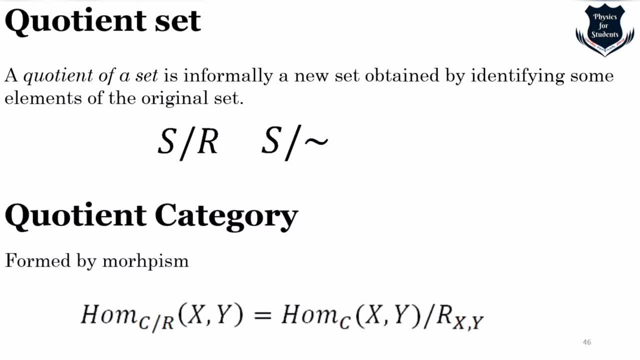 s by or upon three and in quotient category also, it is used using uh, what is called morphism. right now, you might at this point think that what is a quotient set or what is a quotient category, although this video, uh sticks to the basic point, that is, understanding. 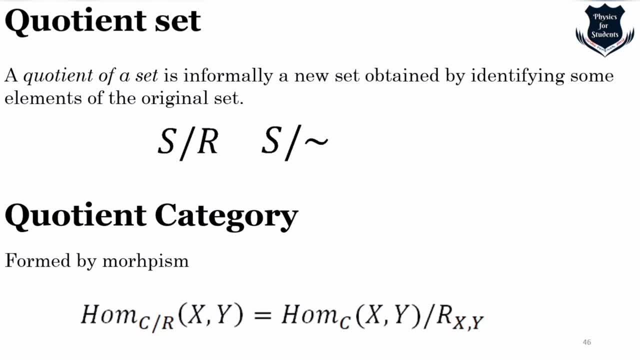 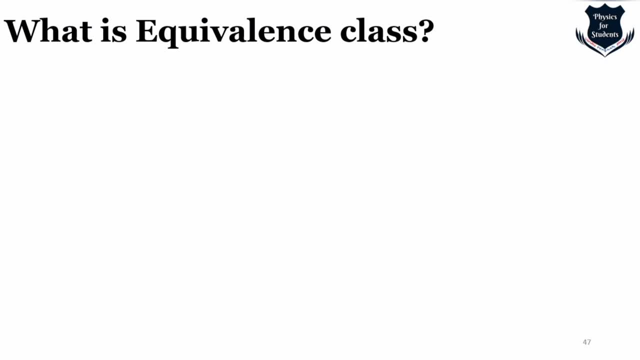 the origin of the symbols. but definitely it is a good point to understand what is a quotient set. i will just go back and make you understand what is an equivalence class first. now you see this figure. it is two triangles which are congruent to each other and these two triangles are not. 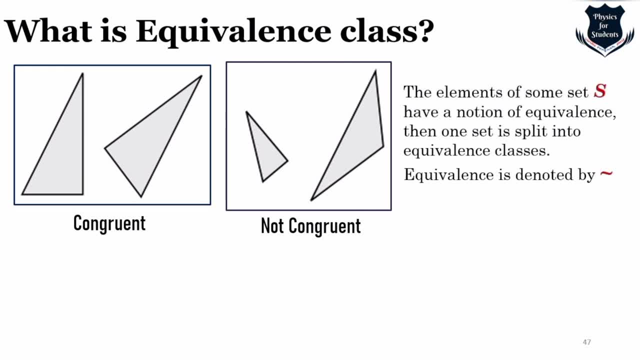 congruent to each other right, and we call them the element of some set s, whichever notion of equivalence. it gets split into equivalence classes and this equivalence is denoted by the equivalent sign, you all know. and this equivalence classes form a partition. i mean to say partition means 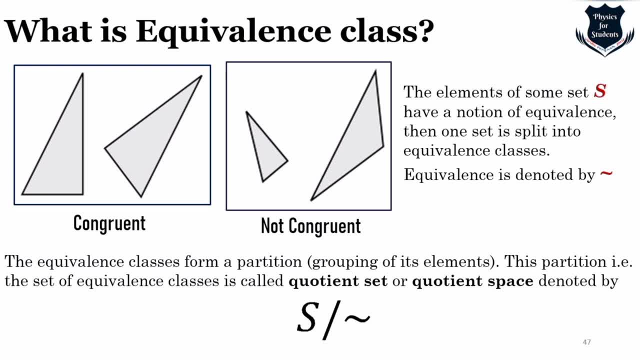 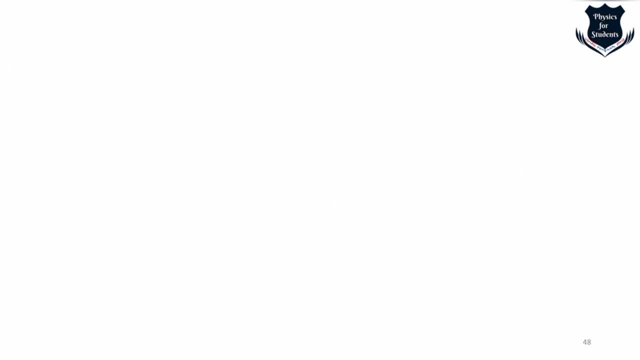 it is grouping of elements. this partition, that is, a set of equivalence classes, is called quotient set or quotient space, and is denoted by this one, which includes a slash sign introduced by al-hasr or abu bakr. now i would like to explain you in easy term now, for example: so these elements have: 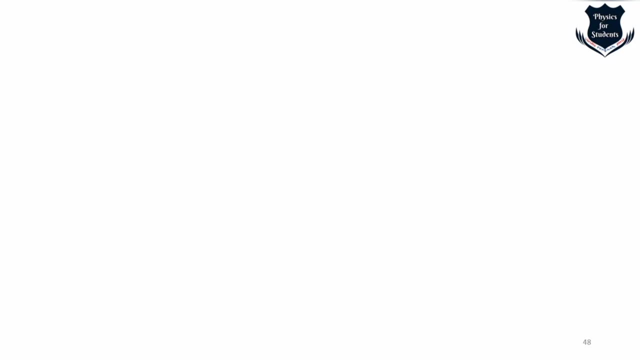 notion of equivalence. you have seen that one may naturally split into others and these equivalence construct the elements. now, for example, we set capital c as a set of all cars, okay, and this one tilde c is an equivalence. we all know that. that means say, for example, it is of the same color. 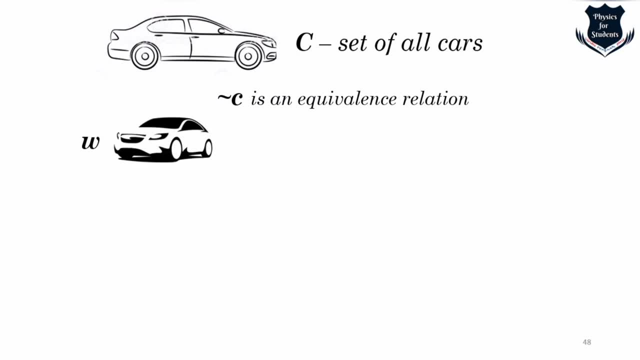 okay. so for some white car which is w and some for other white car which is h, we denote this as this one okay w which has got an equivalency. we have seen that one may naturally split into others and these equivalents construct equivalence in relation with the another class H. So with that kind of an equivalence relation we get. 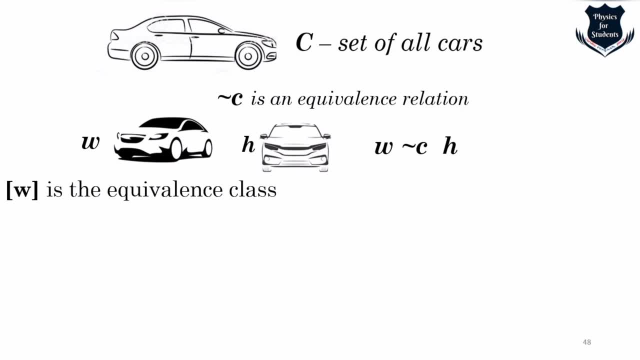 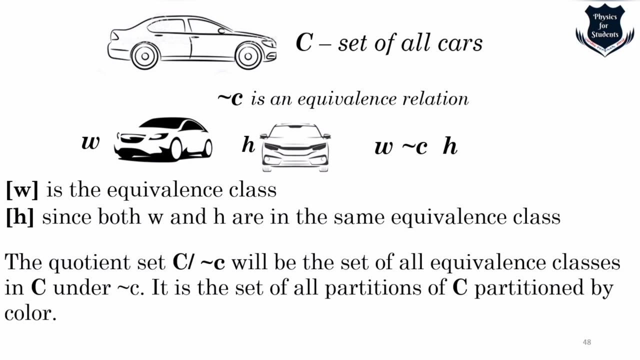 W. it works well because it means the equivalence class right and is the partition. since both W and H are in the same equivalence class, we can write this: So the quotient- this one which you are using for the equivalence quotient set- would be a set of all equivalence classes in C under this one. 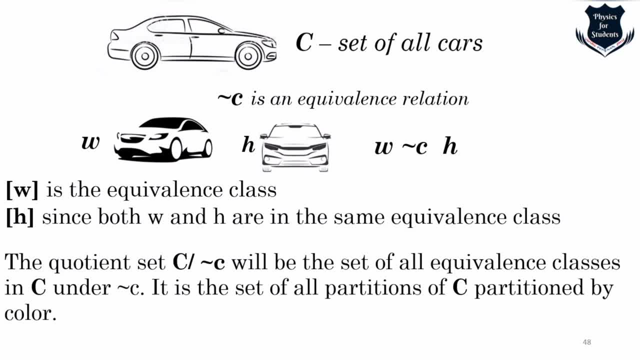 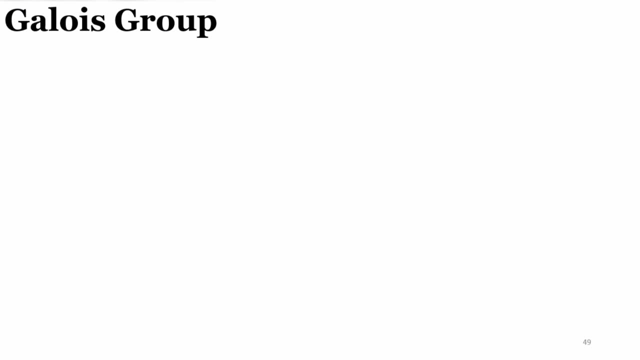 sign, tilde C, it is the set of all partitions partitioned by color. So I think that gives you a basic understanding what do I mean by quotient space and quotient set and what I tried to explain to you earlier. Now, this slash sign is also used in something which is called a. 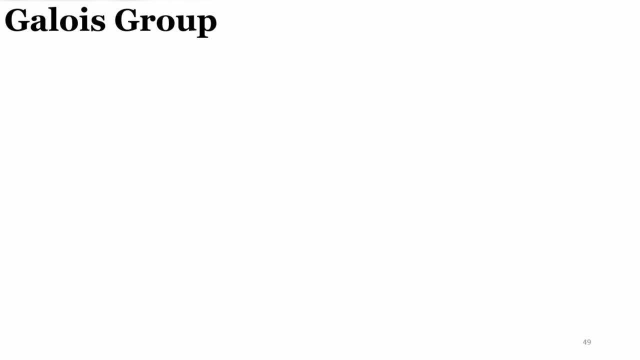 Gallois group. Now, those who are aware about number theory in mathematics, in the area of abstract algebra there is a Gallois theory, The Gallois group- of a certain type of field extension is a specific group associated with the field extension. So suppose that E is an. 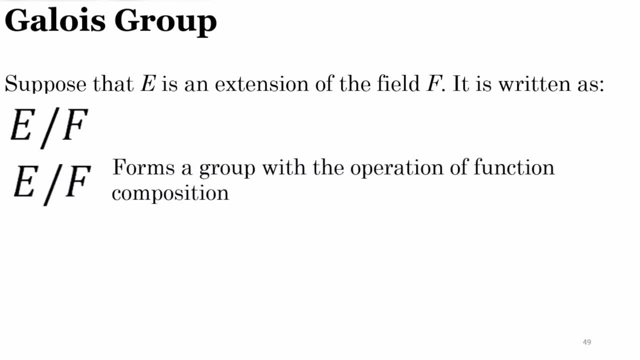 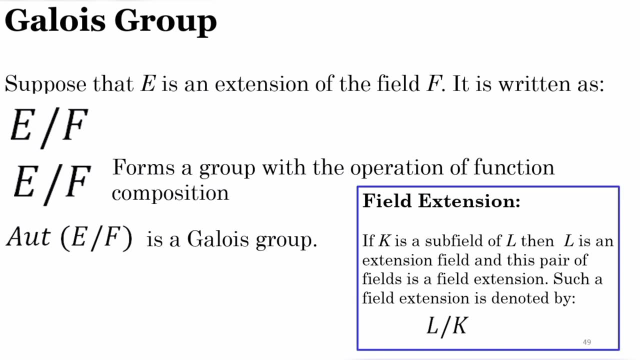 extension of the field F. it is written as this: and E upon F forms a group with the operation of function of composition. it is also called a Gallois group. and on the right hand side I have given what do we mean by field extension, although again it goes much more into details. So study of field. 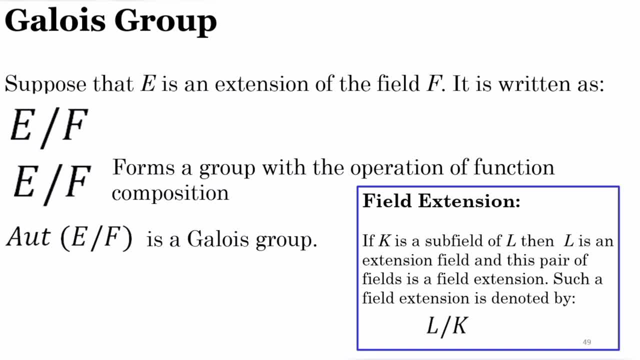 extension and their relationship to the polynomials that give rise to them via Gallois group is called Gallois theory, which I'm not going to explain, and it is named in honor of a very young, extremely talented but a very unfortunate young mathematician, Everesti Gallois. So we come to something which we 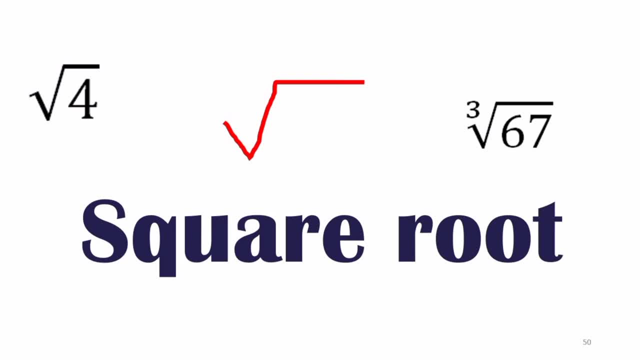 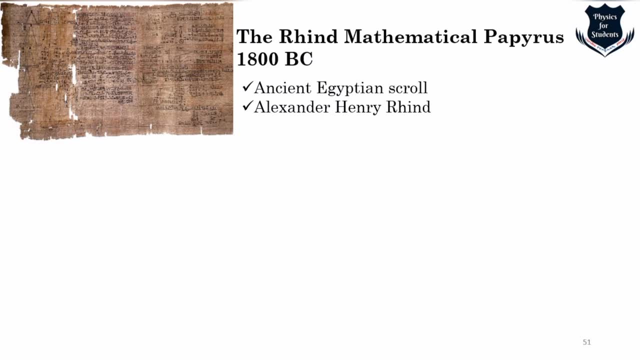 all know. So it is called square root. but this square root has got a very interesting history. Now we all know about what is called this Rind mathematical papyrus. So this Rind papyrus is a famous document from the Egypt, Egyptian Middle Kingdom, and it dates around say: 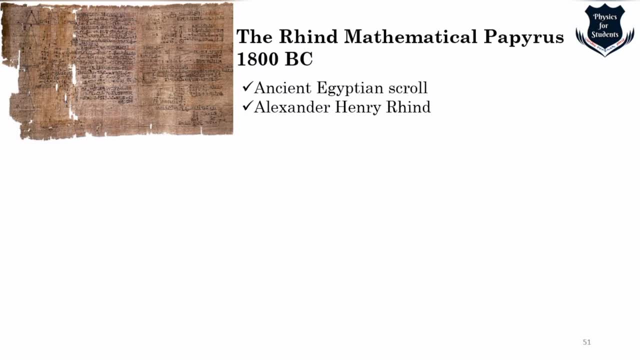 1800- 1650 BC, and it was purchased by Henry Rind in Egypt in 1858 and placed in the British Museum. Now this Y, then we come to what we call is called Yale Babylonian collection. You see this YBC from: 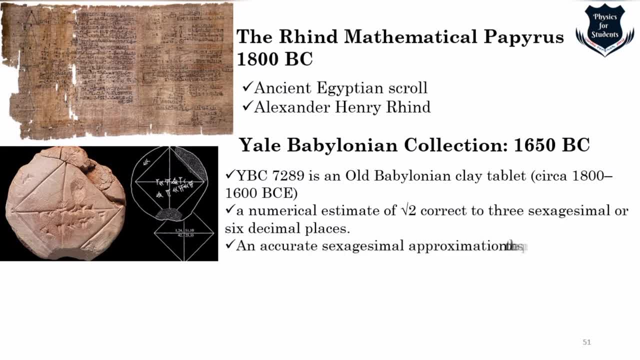 the Yale Babylonian collection is a hand tablet and it appears to be a practice school exercise, which was which was being done during that time by a novice scribe, right, Such an interesting it's. maybe a novice was just scribing on that and putting up some something interesting, But mathematically 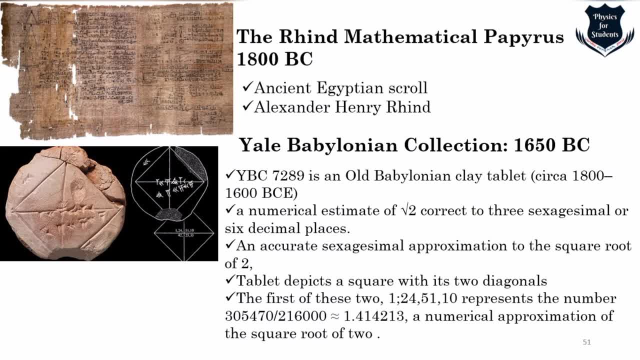 speaking, this second millennium BCE document is one of the most fascinating extant clay tablets, because it contains not only a constructed illustration of a geometric square with intersecting diagonals, but it is also, in its text, a numerical estimate of square root of two, corrected to six decimal or six decimal places. Now the value is read from the uppermost horizontal, If you can see. 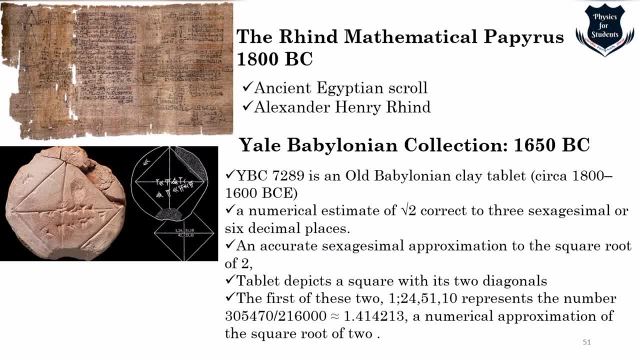 the picture on the left hand side, horizontal inscription, and demonstrate the greatest known computational accuracy obtained anywhere in the ancient world. It is believed that the tablets author copied the results from an existing tablet of values and did not compute them themselves. So, whatever this is, this is something really interesting about the Yale Babylonian collection and 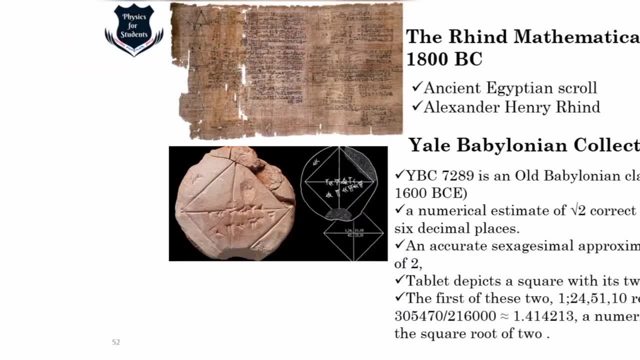 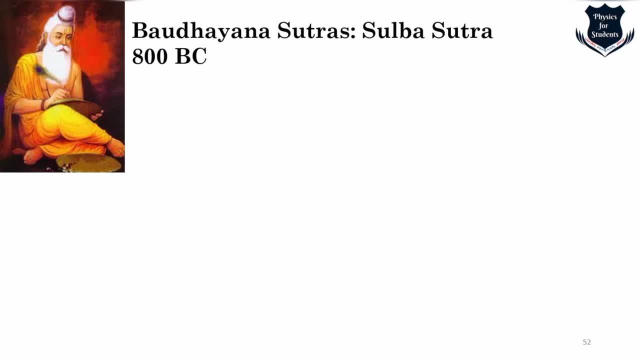 the value of square root of two. But hold on, it is not the oldest one Here. we come back to India, Bodhyayana. well, he was basically a Vedic priest. Now, first of all, let me tell you Bodhyayana Sutras are. 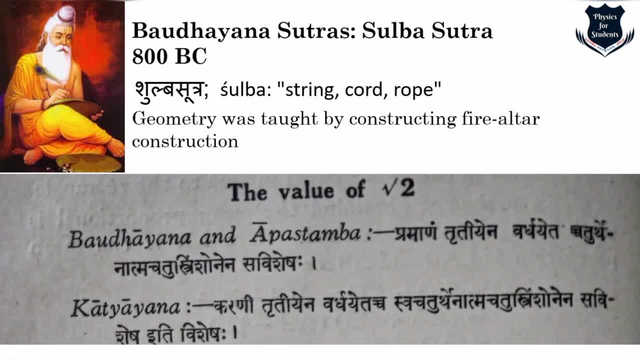 Sulwa Sutras. This one I'm going to explain you later, But first of all let us understand that the geometry during that time, which is quite old, was done by constructing fire altars, So all these holy rituals and the Yagyas doing that Vedic period. This is very important because 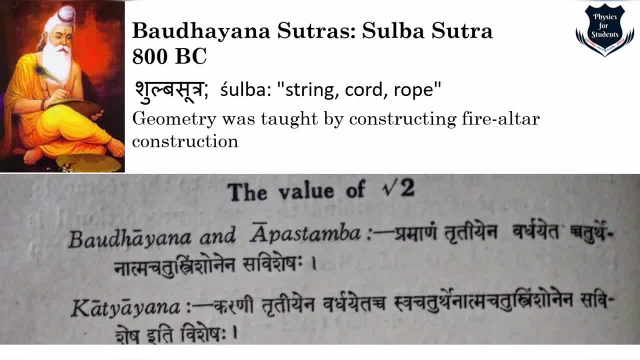 Yajnas during that Vedic period was being done on fire altar. So Bhadhyayana is said to be the original mathematician behind the Pythagoras' theorem. right, I am not going into further argument, but Pythagoras' theorem was indeed known much before Pythagoras. 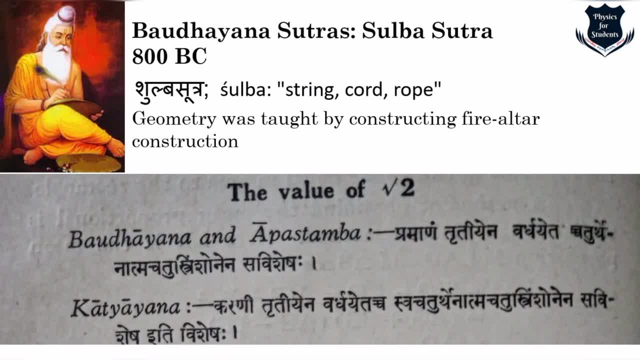 and almost thousand years before Pythagoras was born. So it is widely believed that he was a priest and an architect of very high standards. It is possible that Bhadhyayana's interest in mathematical calculation stemmed more from his work in religious matters than his keenness in mathematics. 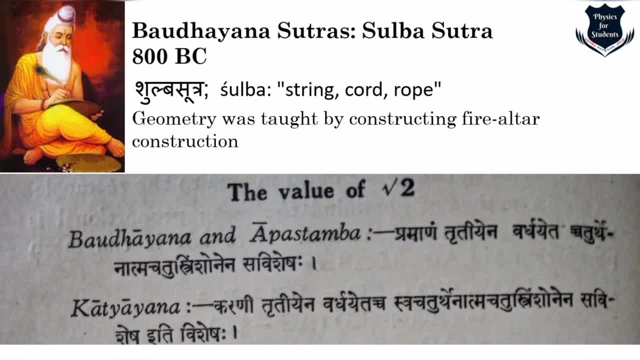 So undoubtedly he wrote the Shulba Sutras. So Sutras means the text okay to provide rules for religious rites, and it would appear almost certain that Bhadhyayana obviously was a Vedic priest. The Shulba Sutras is like a guide to the Vedas. 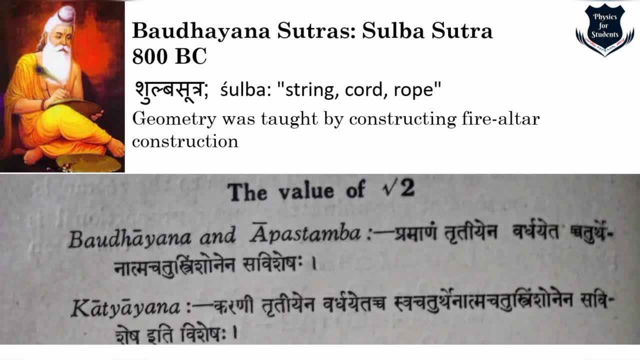 which formulates which I told right on the first, if you see on the screen that it rules of constructing altars and thereby it teaches the mathematics very easily. So the value of square root of 2, it is done by Bhadhyayana. 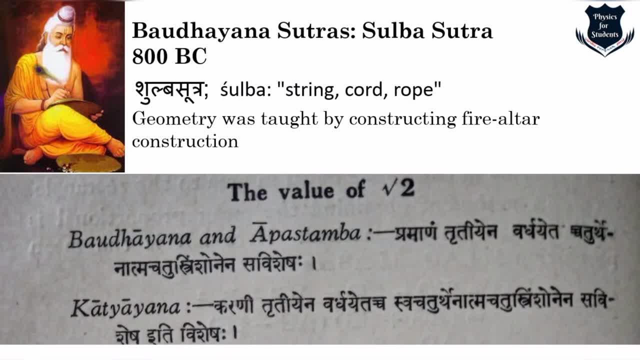 and one of his disciple, Apashtamba and Katayana. It is written in Sanskrit. You can read it out. It says: That means the third part means to increase, And Katayana further says So. if I translate it in English, it comes something like this: 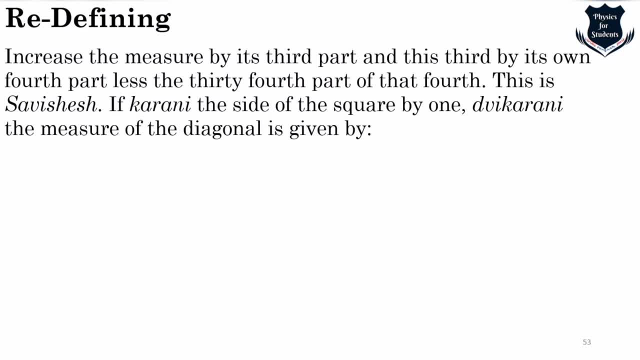 Increase the measure by its third part and this third by its own fourth part, less than 34th part of that fourth. This is Savishesh. So you see, this Savishesh word means Savishesh with Vishesh And Vishesh means Avashesh, Savishesh. 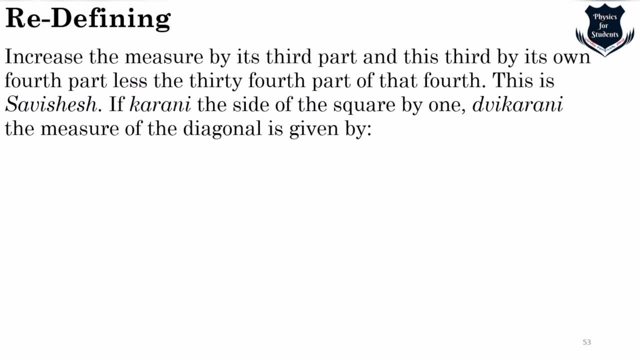 So Avishesh or Avashesh, it means the remainder. So if Karani is the square of Divya, Karani is the measure of diagonal, and here we find the square root of 2.. So this you know, undeciphered, difficult Sanskrit shlokas. 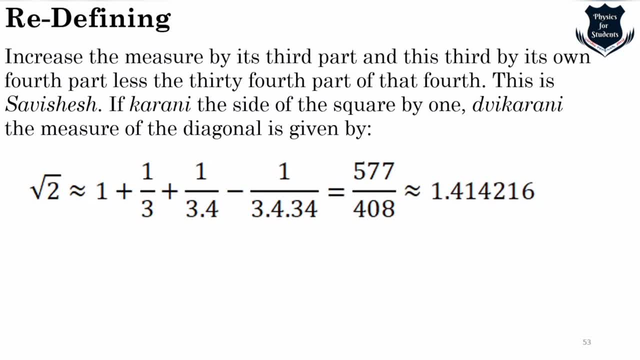 going even further back from Pythagoras' theorem, has taught us to calculate geometry and the value of square root of 2.. But these are so difficult that only the pundits or the elite class knew Sanskrit and was not possible for ordinary mortals to decipher them. 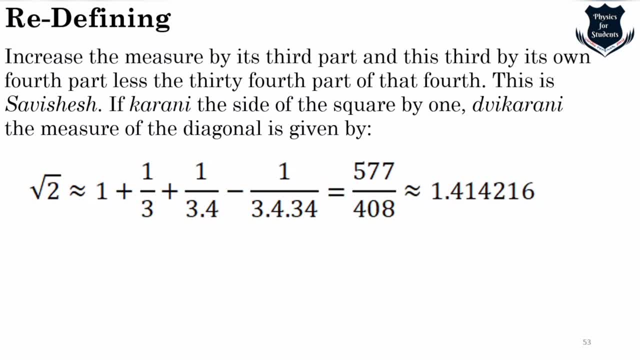 And henceforth it remained something hidden. Bhaudyayana further went and discovered the Pythagorean theorem, the circle of the square and the value of pi. So this is another version which I found. I don't know whether it is right or wrong. 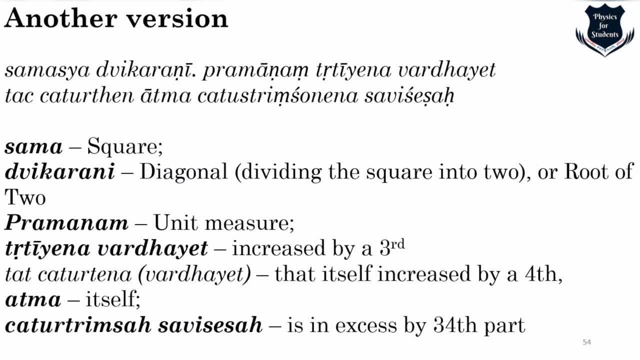 because the previous version I have taken from a very authentic book of my father. My father gave that book and told me this is where it is originally written. So Samaswadvikarena Parmarang Trithayena Vardhayet. 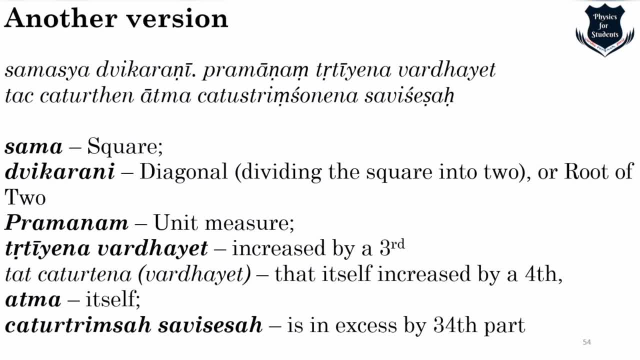 And it seems more or less the verse is to be the same. Sama means square, Divikarani is the diagonal, Pramaram means unit measure. Trithayena Vardhayet increased by third, Atma is itself. 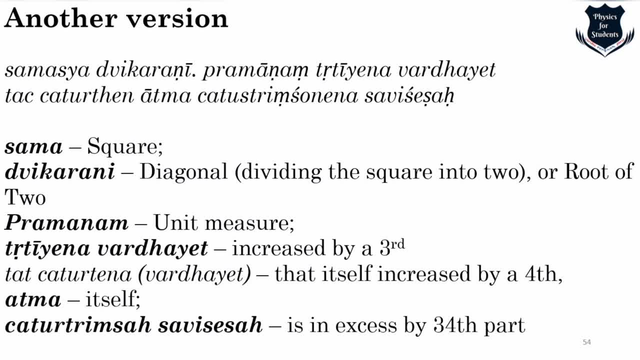 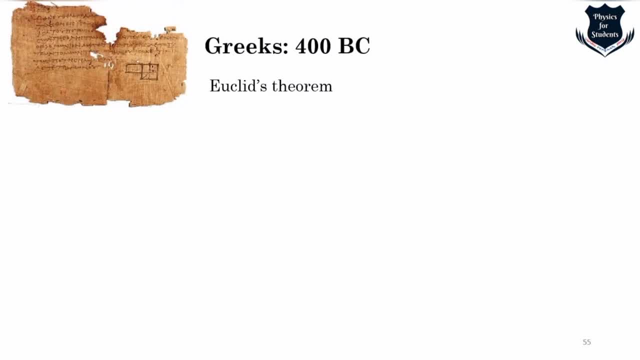 And Chaturstisma Savishes means is in excess by the 34th part. So we see on overall that the Greeks around 400 BC that square roots of positive whole numbers that are not perfect square are always irrational numbers. This is the Euclid's theorem we know. 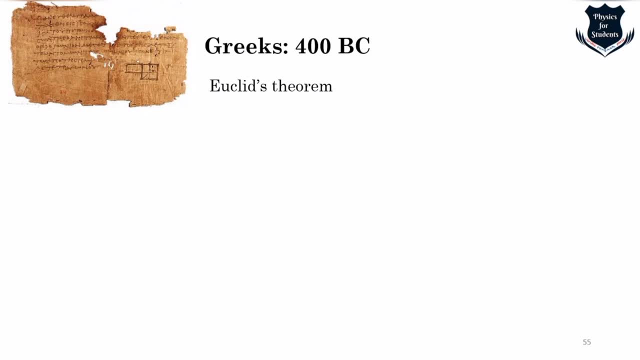 dating back to 400 BC. The particular case square root of 2 is assumed to date back earlier, to the Pythagorean, which is exactly the length of the diagonal of a square of side of length 1.. Then we find Chinese mathematicians around 200 BC. 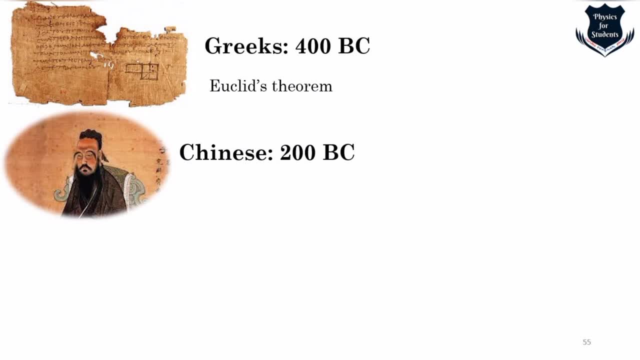 who worked on what is called excess and deficiency, which says to combine the excess and deficiency. as the divisor and the numerator multiplied by the excess denominator and the excess numerator times the deficiency denominator. combine, them becomes the dividend. We also saw that Mahavira, around 800 AD, gave the square root of a negative number. 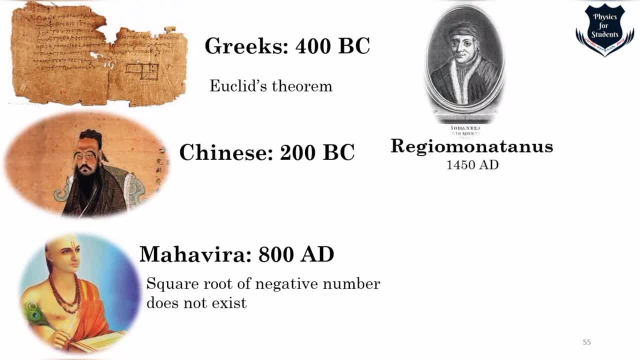 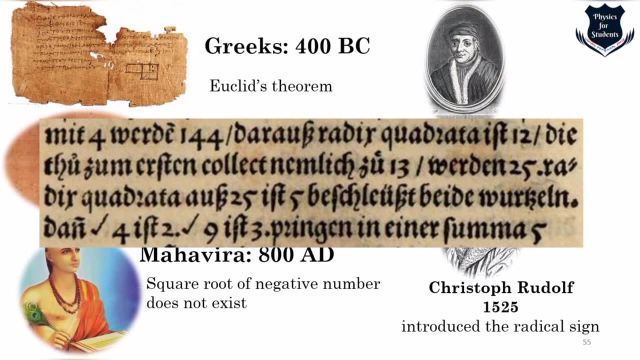 which does not exist. And then, in 1450, the symbol of our square root was invested by Regiomontanus and an R was used for radix to indicate square roots. And finally, Christoph Rudolf, in this book, as you can see right on your screen, 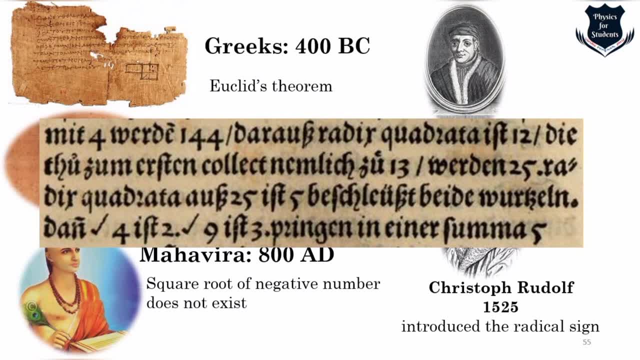 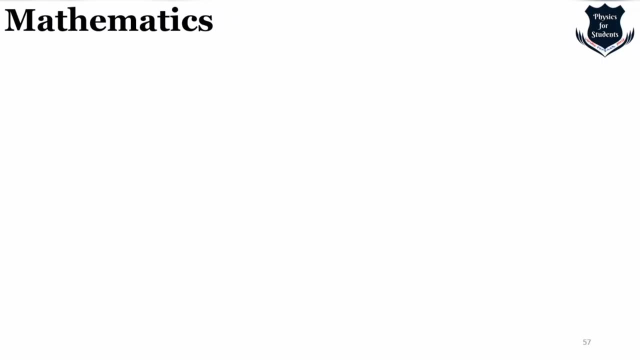 the symbol of square root was first used in 1550 BC. In 1525, and this is an excerpt from the book which you can see, right at the last line, how the square root of 2 is being used. Coming to the last part, which is the exponential in mathematics, 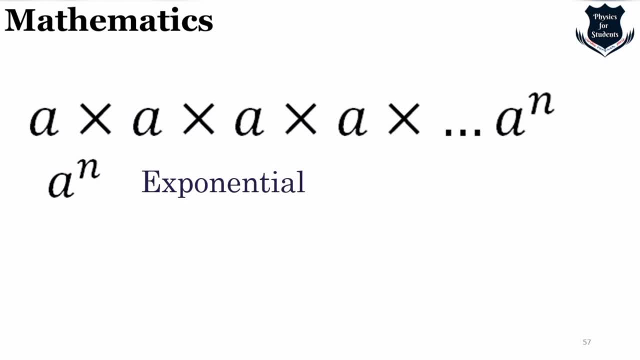 exponential. we all know. a multiplied by a times a times a give rise to a to the power n, And it is denoted a. to the power two, It is denoted as a two and logic, We denote it as and So. 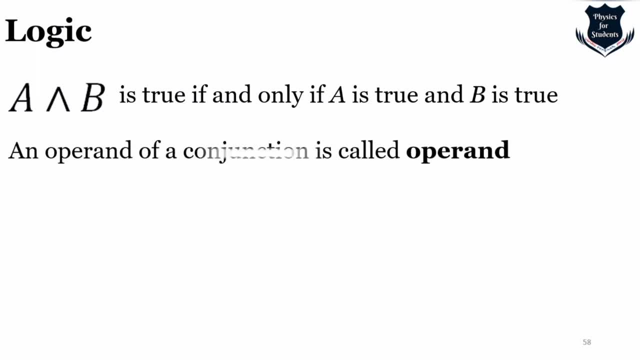 A and B is true if, and only if, A is true and B is true, An operand of a conjunction we know is called an operand, So we say P Joe, it's Maggie and Q marry drink soda, So we call P and Q. 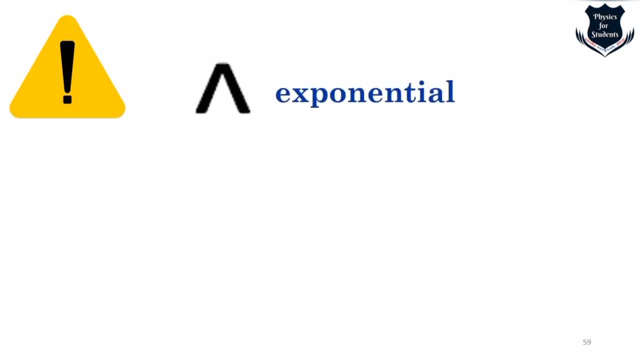 But hold on. Here is also a point of attention. This is an exponential and this is a logical and right. So you see, there is a difference. Those who are aware about using the symbols in equations- it can be latex, or you know. 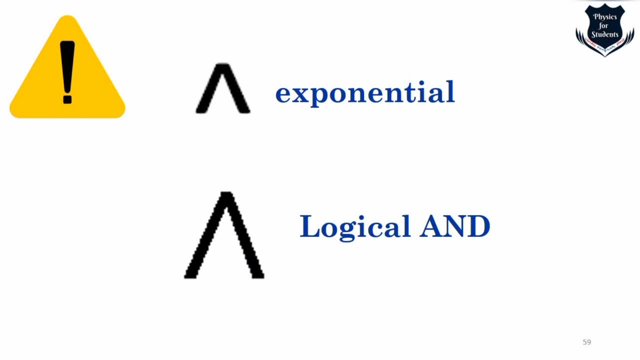 symbols in MS word. You will see these are not the same sign. So, just as dot product and the circle one, which is the composite function, are not the same, The exponential and the logical and are not the same, You see the exponential is a less and the logical one is a bigger one. 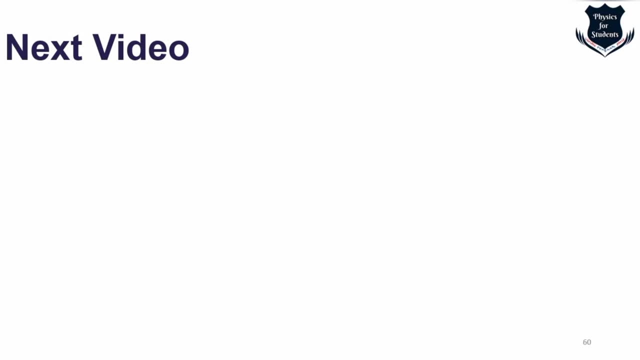 So that's it. I think that we have covered the basic arithmetic operators and the history behind that: Who invented and what are the usages And the common, frequent confusions which arises from the site. So the next video I would be covering on equality, equivalence and similarity. 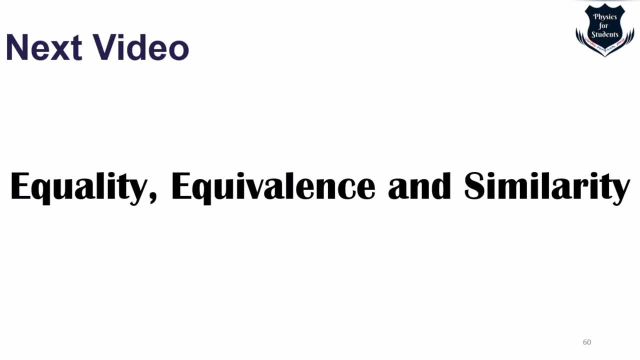 This is equally interesting and it carries fascinating stories, Greek hydrographics and a lot of other things which I'm sure you're going to enjoy. So I would wait for your comment, because this is a new series which I'm starting. Do comment, do like, do subscribe and please let me know how did you liked it, and I would be coming up with the next video.